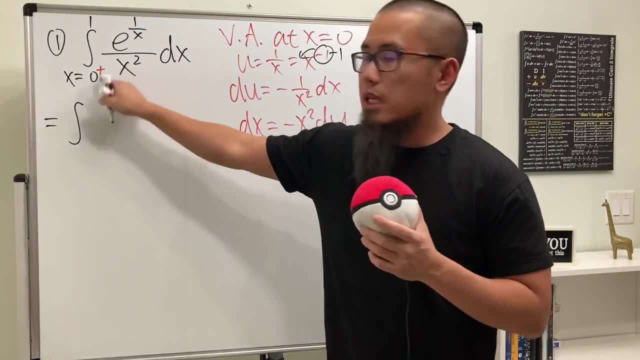 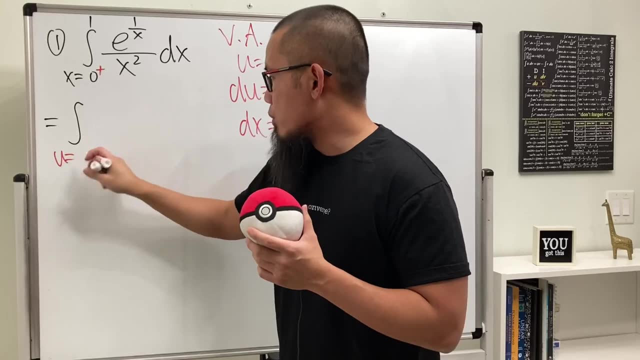 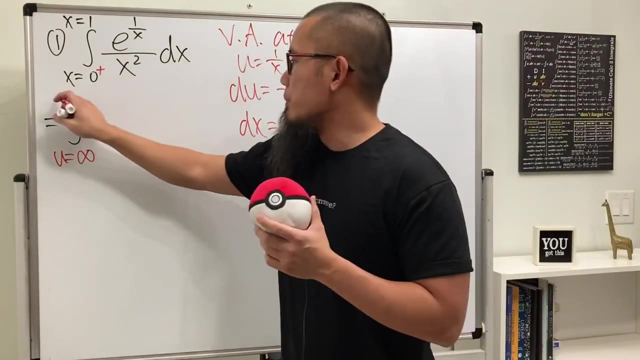 the integral. This is when x is approaching 0 plus. If we put that right here, 1 over 0 plus is positive infinity. So u will approach positive infinity here. And then when you put 1 in here, 1 over 1 is just 1.. So u will be going up to 1.. Hmm, this is kind of weird, because this is bigger. 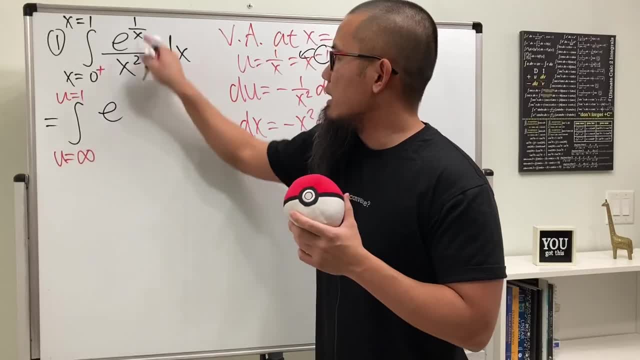 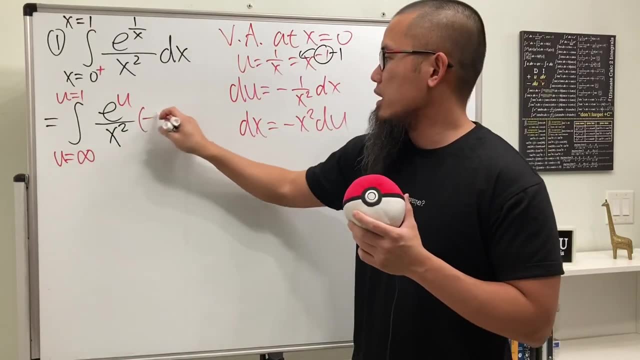 than that. But don't worry, Check this out. Here we have e, And then 1 over x is our u over x squared, And then the dx is that which is just negative x squared du. And this is so nice because 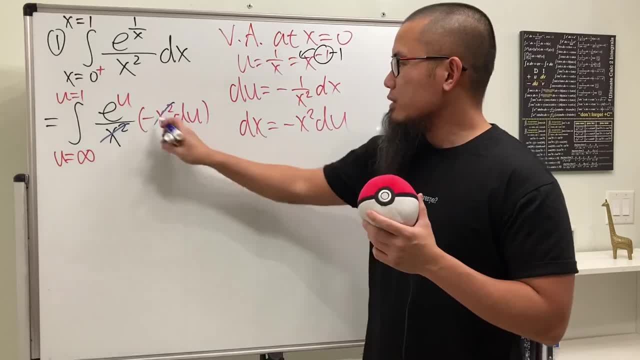 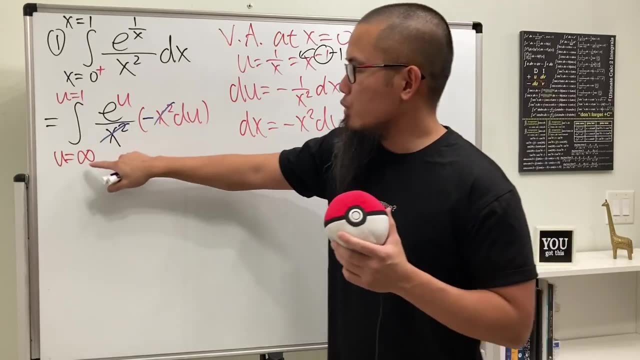 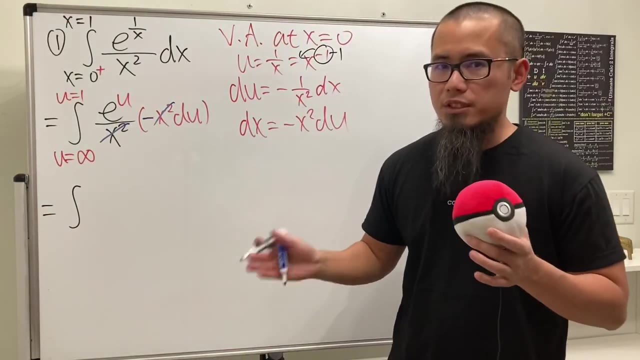 x squared, x squared, cancel out. And you see we do have the negative And, just like what we did in the previous video, we can actually use this negative to switch this and that right. So I'm going to just write down: We will be integrating And, of course, we can finish everything in the 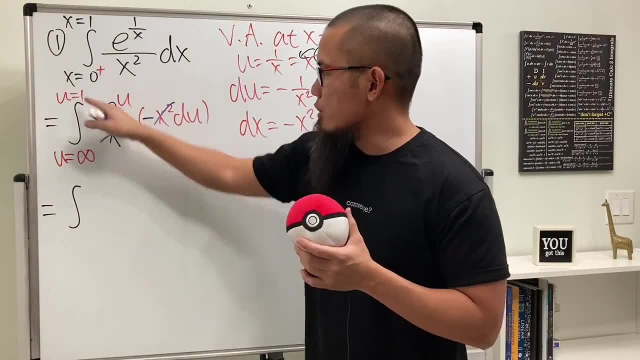 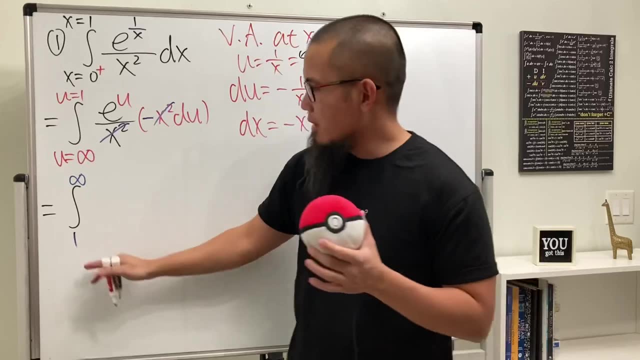 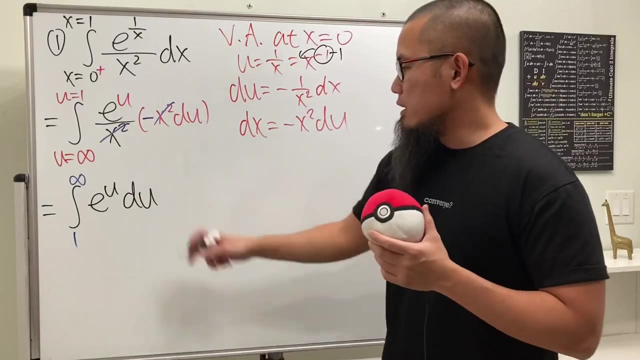 u world, And again I'm going to use this negative. I will just put down 1 here And then infinity here. Ah, that's the order that we like, right? The small on the bottom here, and then the top one should be bigger, All right. And then we have e to the? u du, And you see, right here. 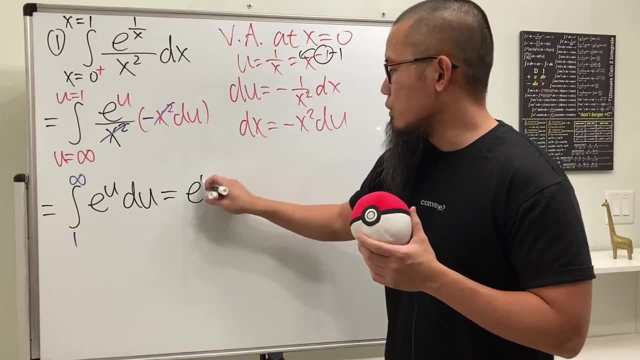 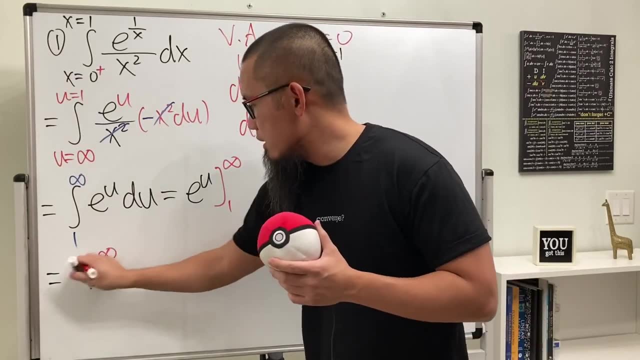 we'll just have to integrate e to the u in the u world, which is just e to the u, And then plug in, plug in right, And you see, when we plug in infinity, we get e to the infinity and then minus. 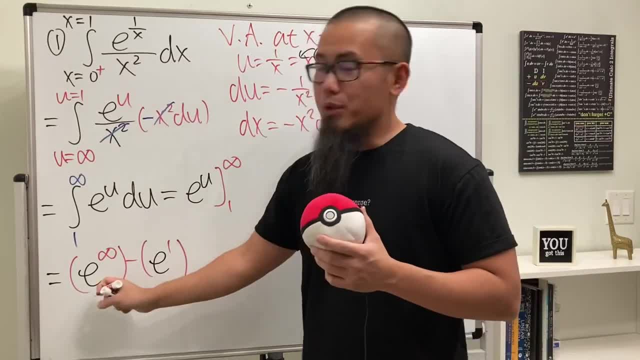 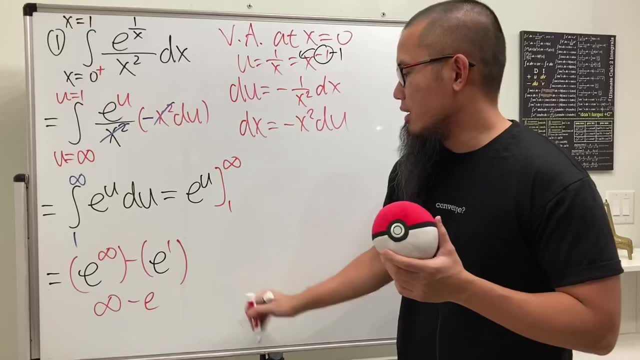 the second term, which is e to the 1. e to the infinity is just infinity, And minus e to the first is just e, which is finite Infinity. minus e is still infinity. So, as you can see this right here, it's infinity. But perhaps we'll just say this: integral diverges. 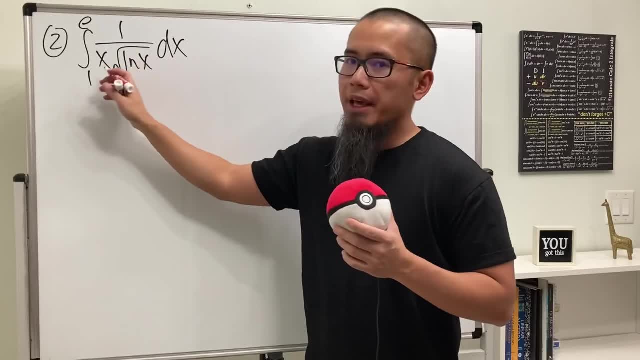 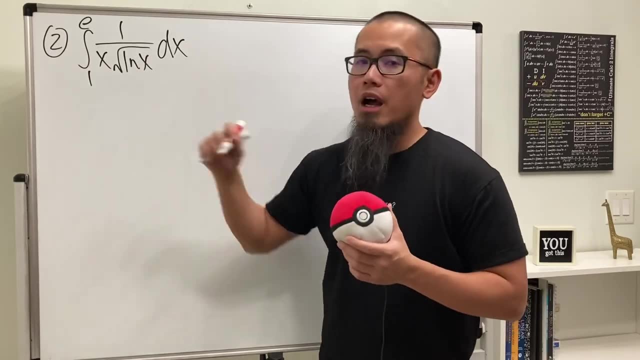 For number two, we have the integral going from 1 to e of 1 over x times square root of ln x. So where is the vertical acetone 1.? Because when you put 1 inside here, ln 1 is 0. And that will make the whole bottom 0.. Yeah, So here let's go ahead and just indicate. 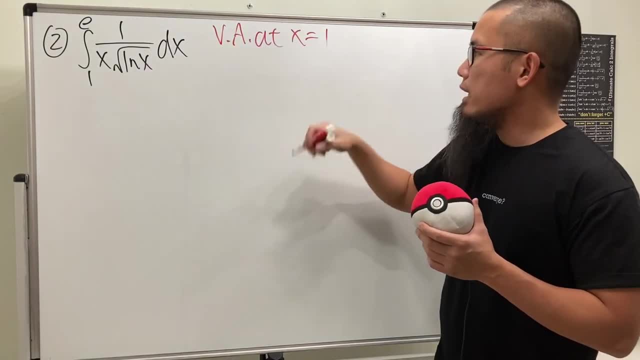 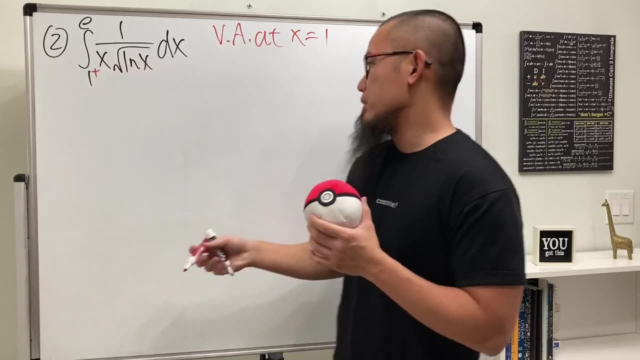 that we have a vertical acetone at x equals 1.. And of course we can take off this easily with u sub. And again here this is technically 1 plus then, Because again we have to avoid exactly 1.. 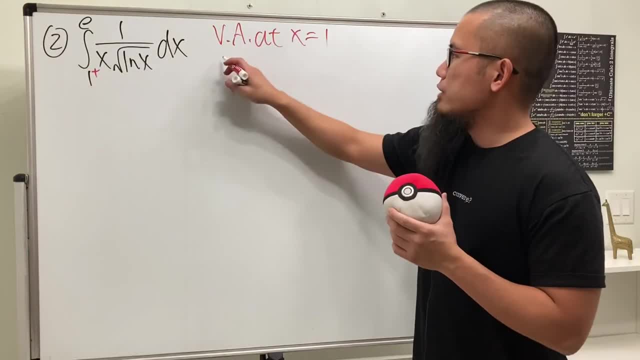 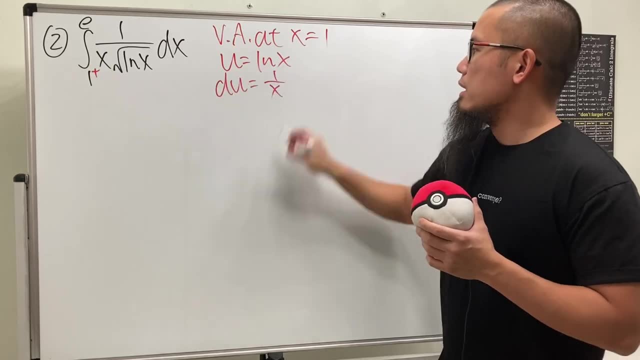 Take the limit. That's the idea. Anyway, let's go ahead and just do u sub, u equal ln- x, And then we see that du is just equal to 1 over x- dx. So you do see the 1 over x and the dx right here. 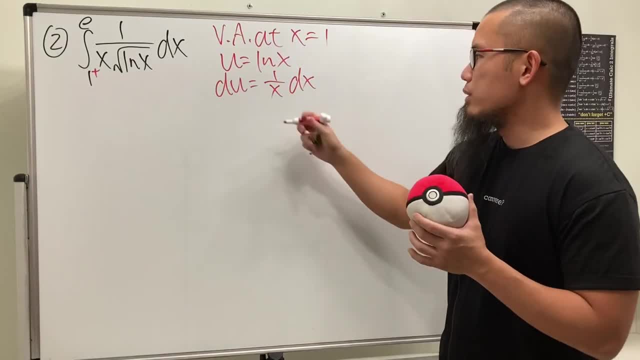 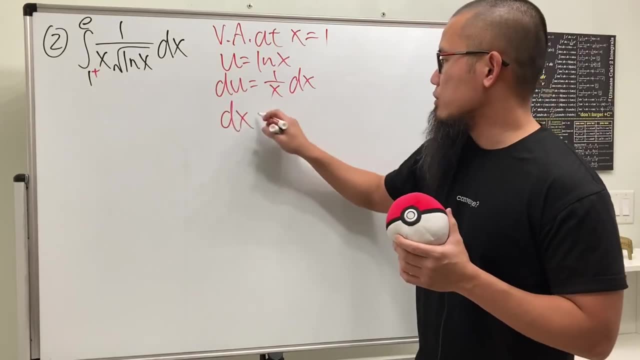 So, if you would like, I can actually just repeat this. So we have a vertical acetone at x equals 1. Right away. Or, if you would like, you can also just multiply the x on both sides So you can see the cancellation. So it's up to you. Perhaps I'll just show you guys the cancellation. It's. 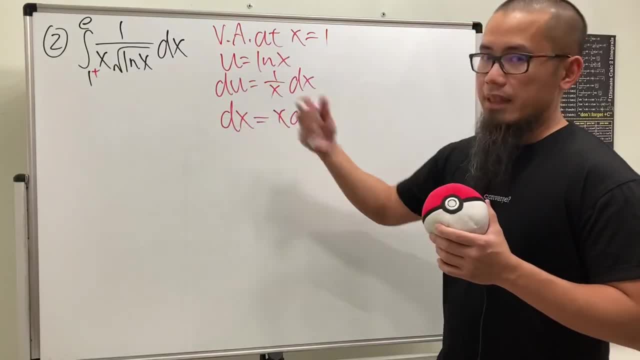 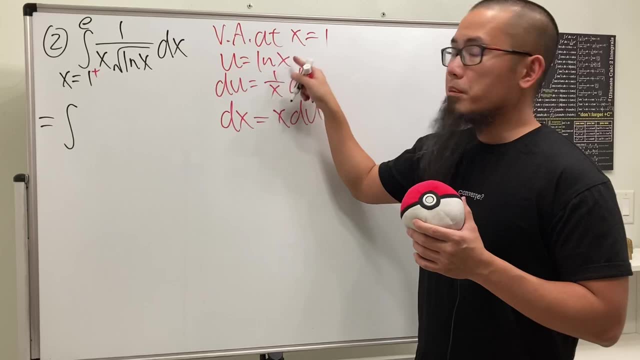 not bad. Multiply the x on both sides like this. And now take this integral to the? u world. Well, this is, x is approaching 1 plus. You put it here: ln 1 plus is 0. But it's a little bit. 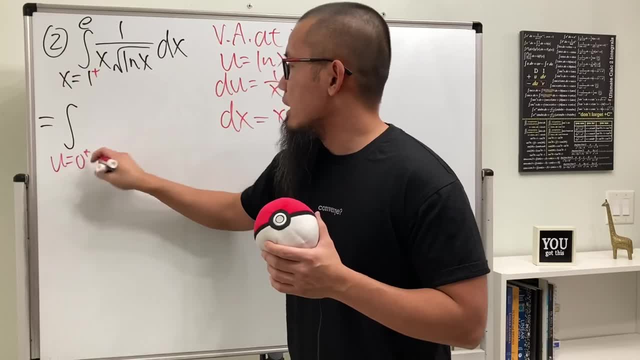 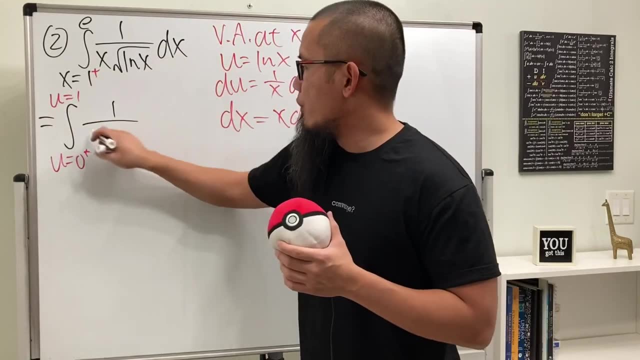 bigger than that. So it will be 0 plus. And then if you put e in here, ln e is 1.. So it's just 1. Right here. And then here we have 1 over x square root. This is the u And this is x du. And I told 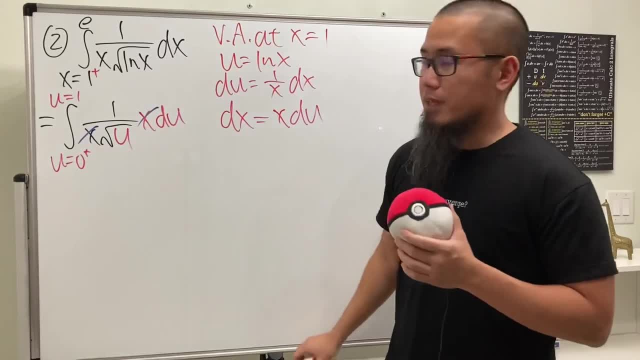 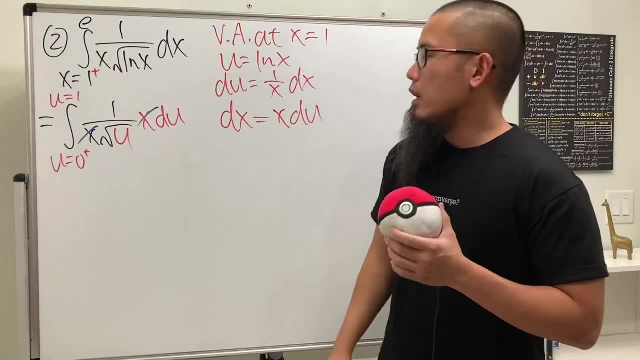 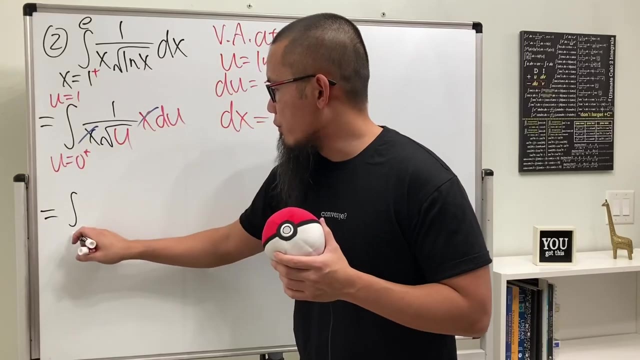 you, we can just have this and that cancel. So if you really want to skip this step, it's totally okay, Because 1 over x dx, that is exactly the du. But anyway, we will integrate this And again we'll finish everything that you world, And to do that, we are looking at the integral from 0 plus. 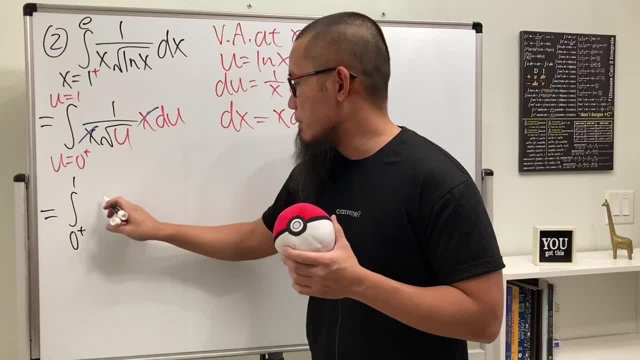 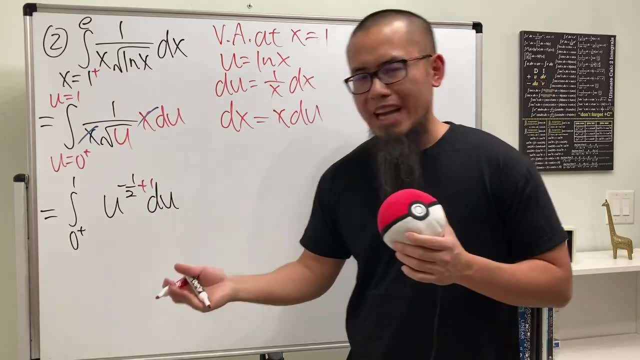 to 1.. 1 over square root, that's the same as u to the negative 1 half power in the? u world. add 1 to the power- negative 1 half plus 1 is positive 1 half- and then divide it by the new fraction right new power which is going. 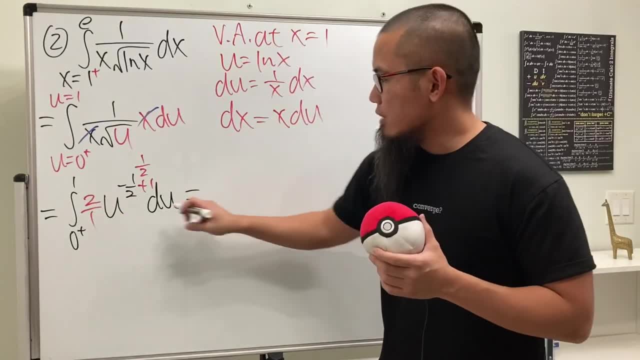 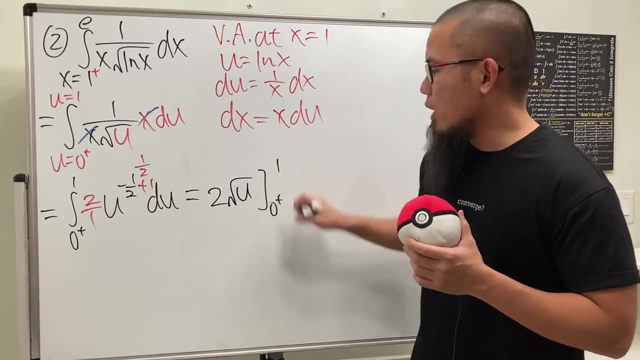 to be multiplying by 2 over 1. so we get 2 and then u to the 1- half is the same as square root- and then we have the u and then we go from 0 plus to 1. plug in, plug in. so the first term is: 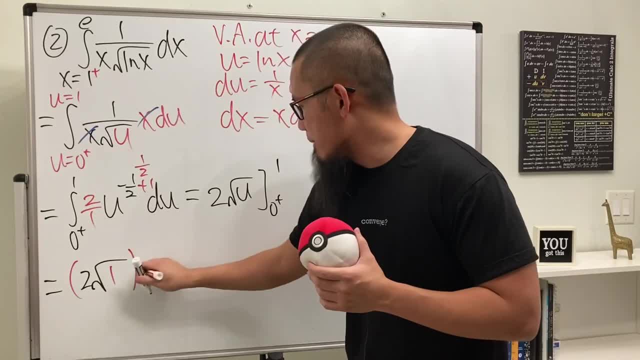 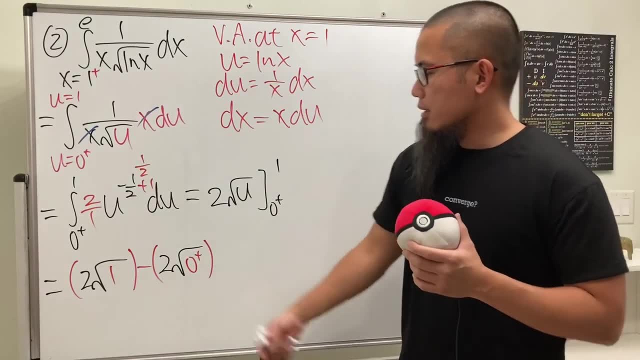 2 square root of 1 and then minus, put a 0 plus. here we get 2 square root of 0 plus. all right, this right. here is just 0, that's just 2. so altogether we just get 2 and this right here. 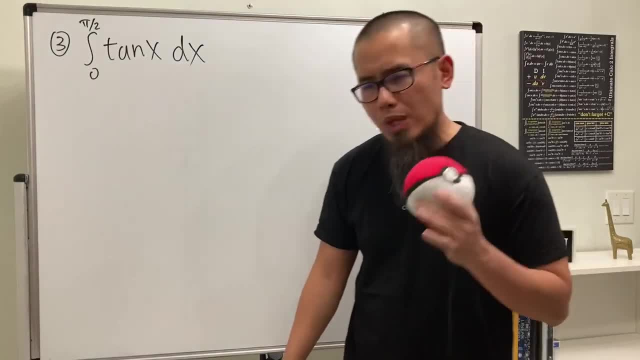 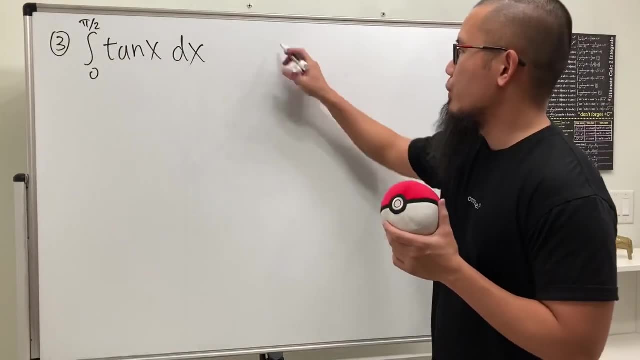 converges to 2, and then we have that number 3. we are going to take care of the integral going from 0 to pi over 2 of tangent x. well, let's take a look at the graph of tangent x real quick. let me just remind you guys, we have a vertical acetone. 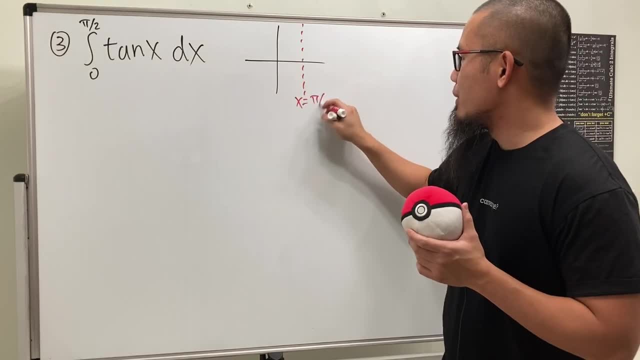 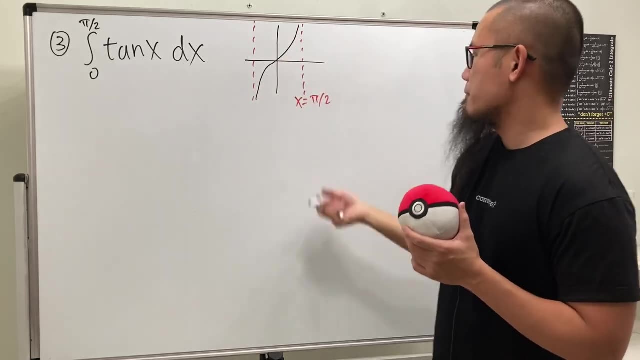 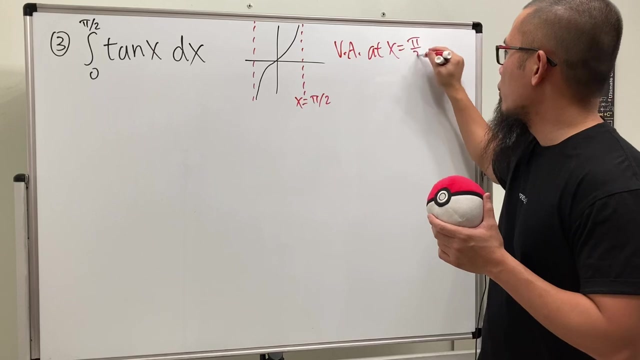 at pi over 2. so that makes this improper, because if you take a look, this is the graph for tangent x. it goes like this, right? okay, so let's just go ahead and just write this down real quick: vertical acetone at x equals pi over 2 and technically we will just have to integrate. 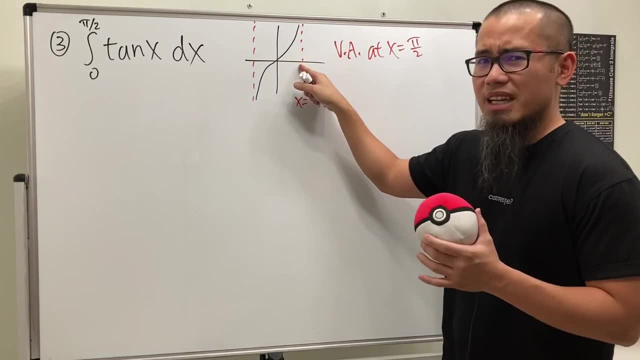 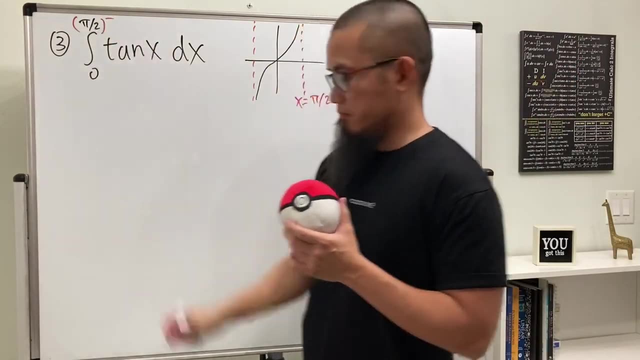 from 0 and then stop right before right. but that's the idea of taking the limit approaching pi over 2 from the left hand side. so this is an integral like this with a minus. so just keep that in mind once we do the limit that would be. 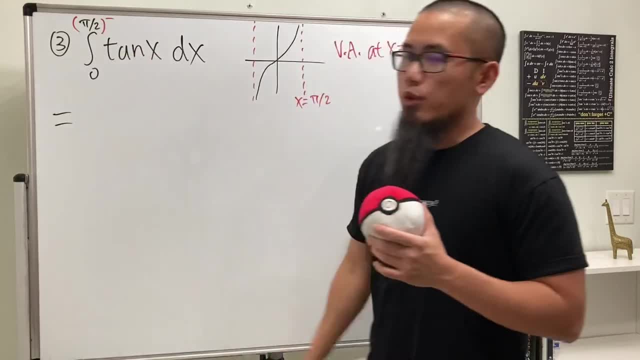 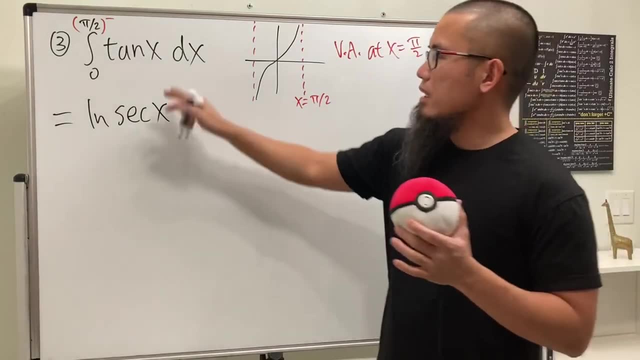 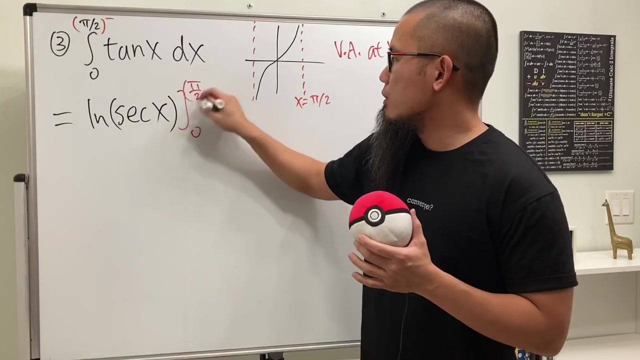 helpful. all right, so we know the integral of tangent x. we have did that many times- is ln absolute value of secant x, but the inside will be positive. so you can just put out parentheses and then we just have to go from 0 to pi over 2 minus, plug in, plug in and see what happens. 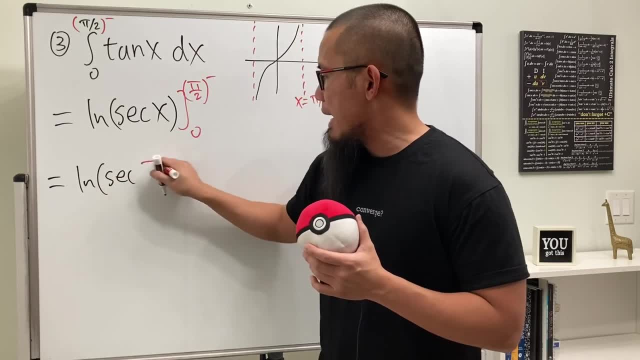 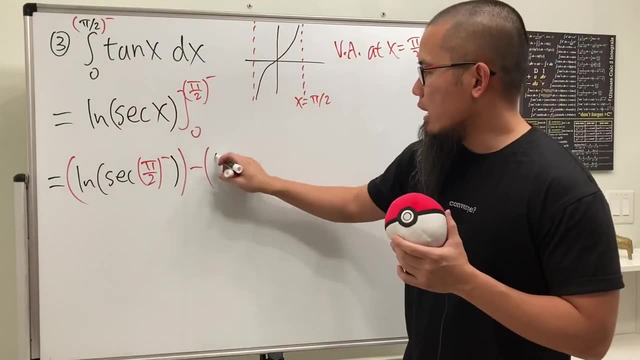 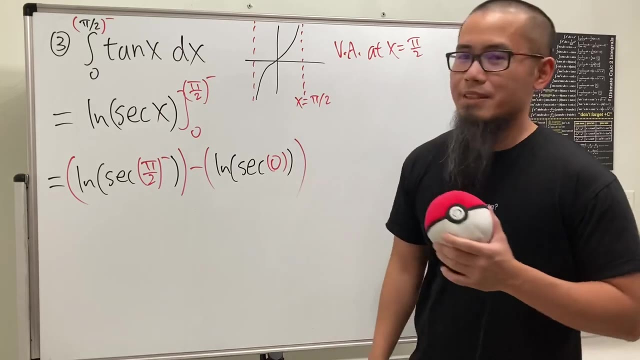 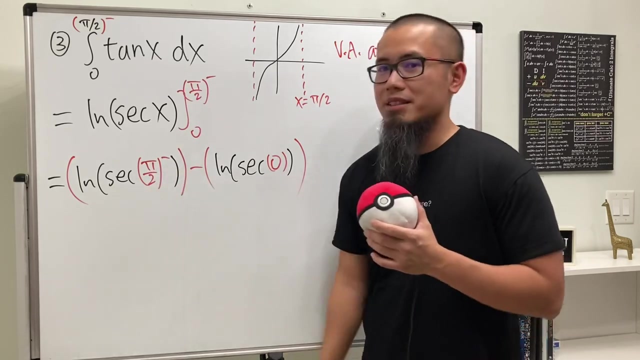 so the first term is ln secant pi, pi over two minus and then minus. the second term is plugging zero. so we get ln- parentheses, secant zero, and then parentheses, and then parentheses. All right, now, this is the part that's going to give us trouble. Let's talk about what secant pi over two minus is. So if you look, 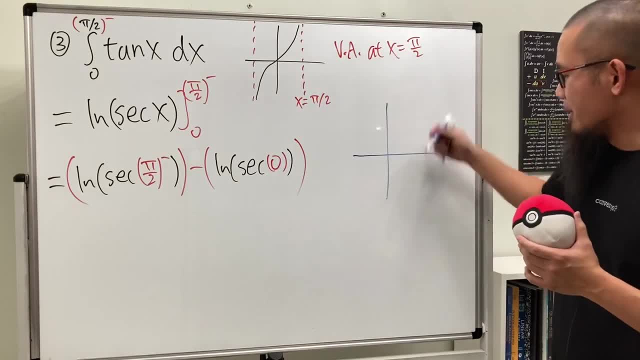 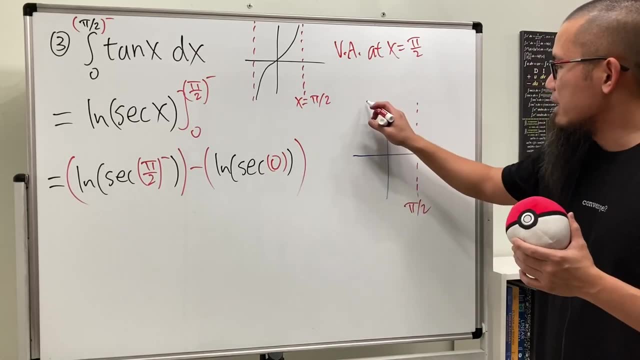 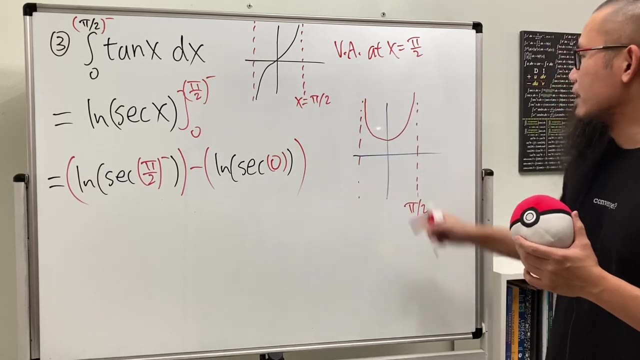 at the graph of secant x again. this right here also has vertical acetone, So I'm just going to put on a dashed line like this: This is a pi over two and secant is a reciprocal cosine, and the graph looks like this, like a u, and then the other one's like this: right, So open up u, But anyway. 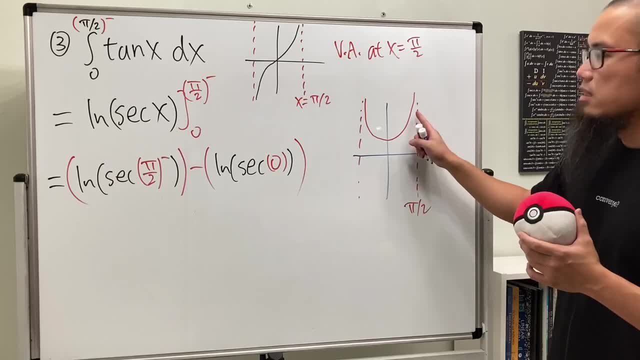 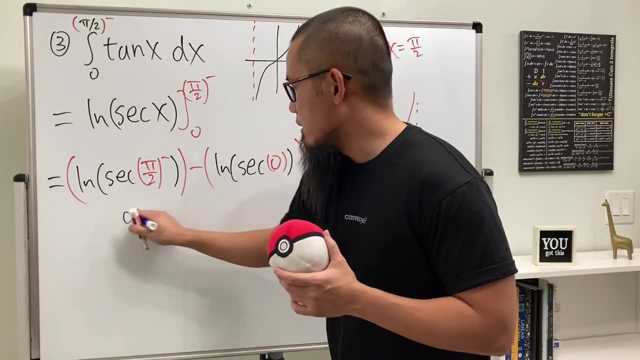 though you see that if we approach pi over two from the left-hand side, secant x is going to go to infinity. So this part is going to be infinity, and we see that we just have infinity here. and if you do ln of infinity, that's still going to be infinity. 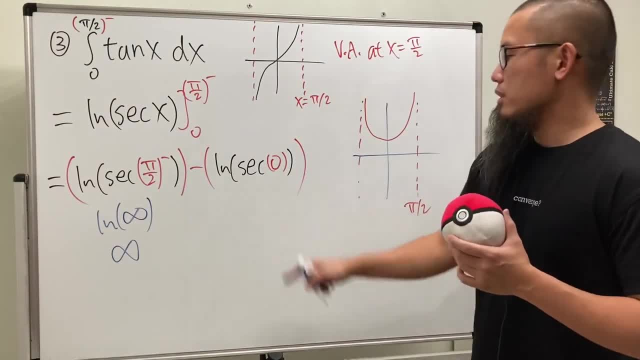 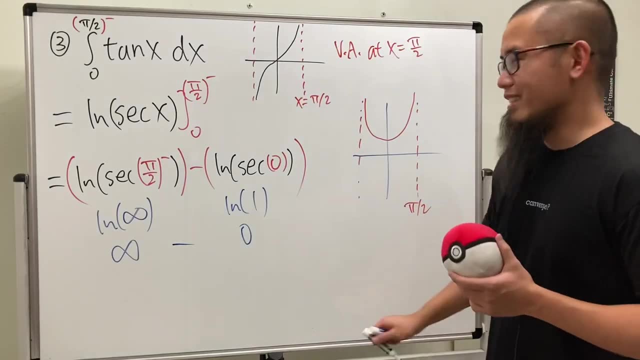 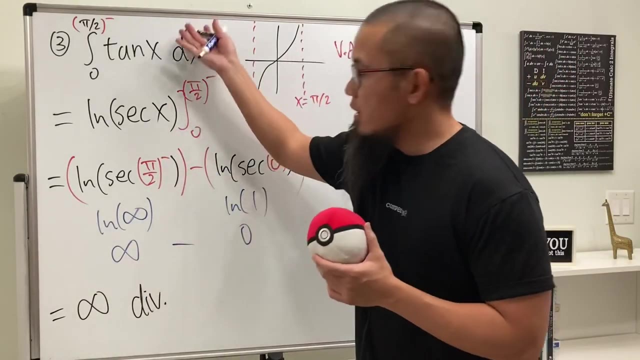 to be infinity. what's secant of zero is just one, and then l and one is just zero. so we have infinity minus zero. so you know it's gonna be infinity. right, the whole thing is infinity. and of course we can just say this: improper integral diverges number four. we have the integral going. 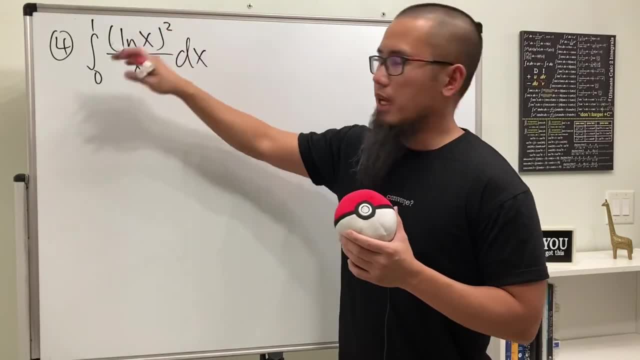 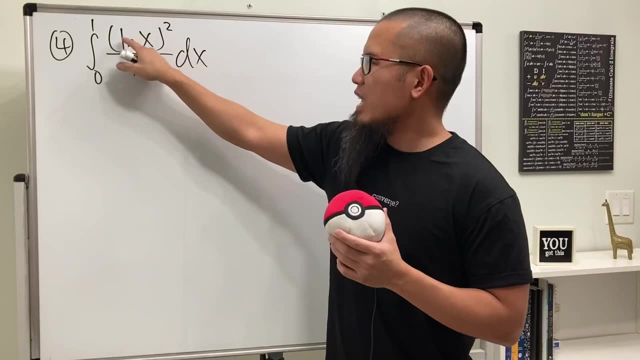 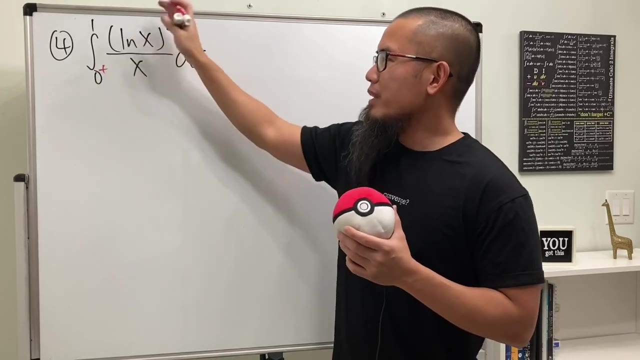 from zero to one of ln x in the parentheses, and then square and then divided by x. first off, when x is zero. this is going to be crazy on the top. inside here we get negative infinity. if x is approaching zero plus right and then square. that is infinity over zero plus you just have a vertical. 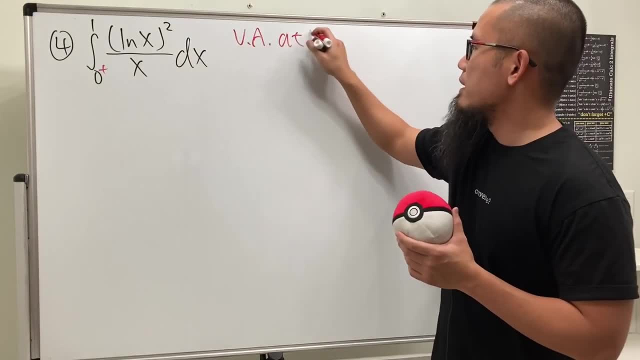 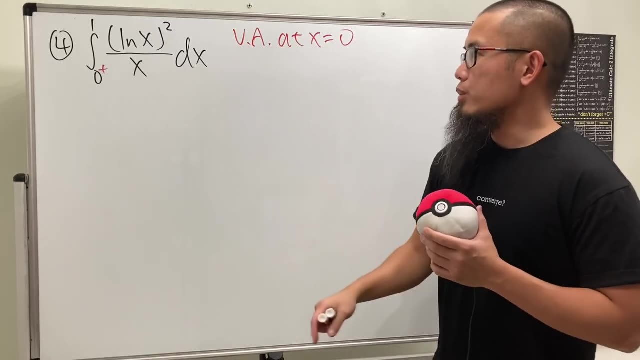 isotope. so let's go ahead and just write that down real quick. vertical isotope and x equals zero. same thing, right, we do the zero plus, just like what we have done earlier, and for this one you do not have to use integration by parts, we can just do use up, if you. 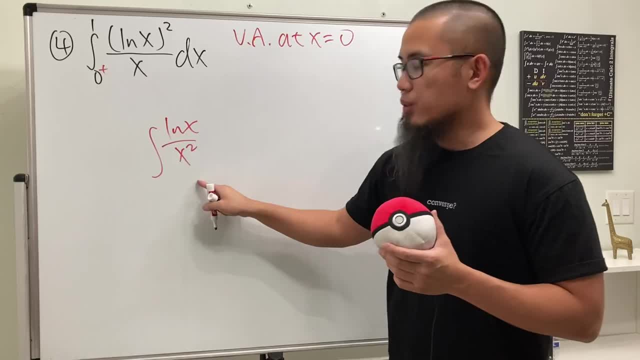 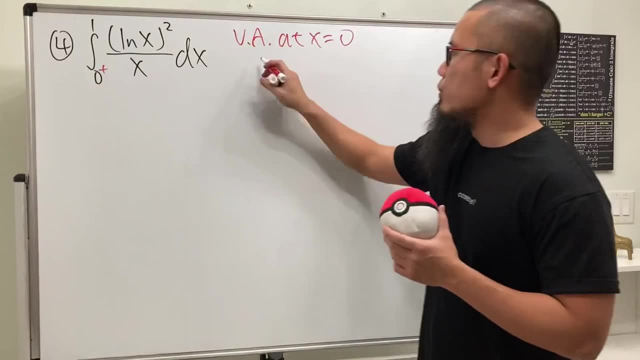 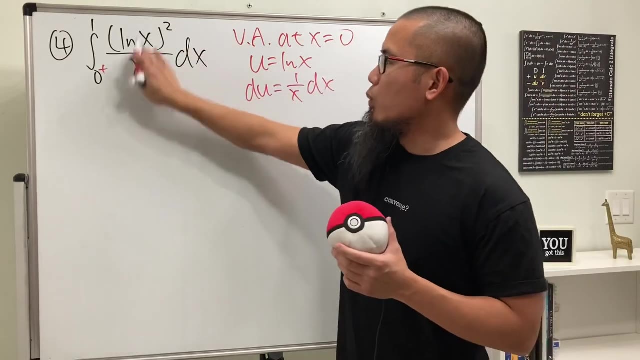 have ln x over x squared. this integral- you know it is integration by parts, but for this one we can actually just do use up, because we can let u equal ln x and then du is just equal to 1 over x dx and you see that we have the 1 over x dx already. so this right here is really just to integrate. 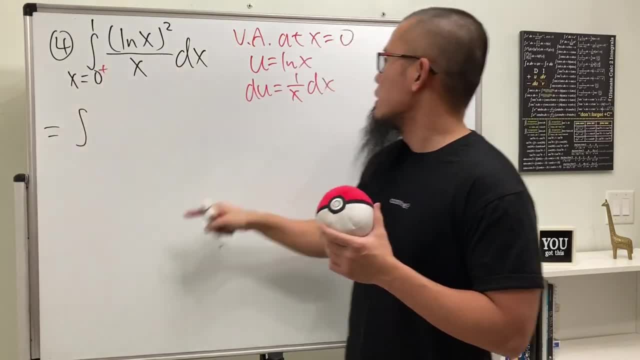 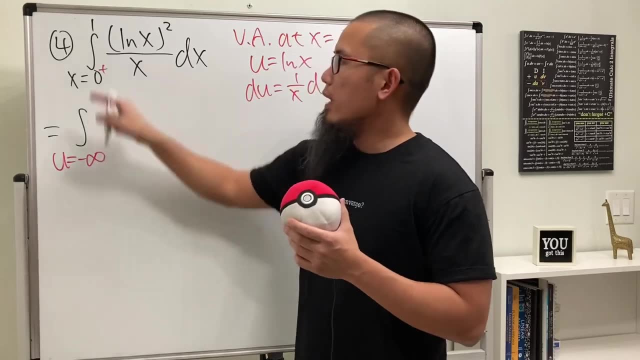 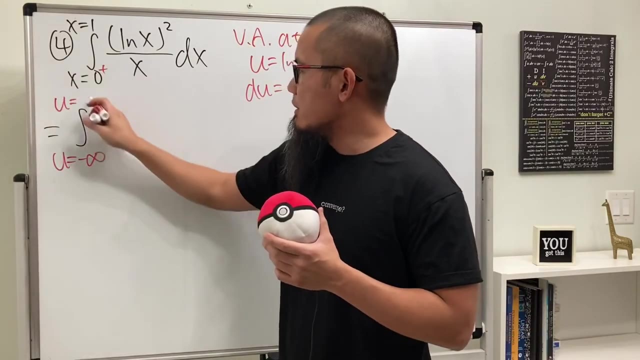 and now when x is 0 plus, you put it here: ln 0 plus is negative infinity, so u will approach negative infinity. and when x is 1, you put it here: ln 1 is 0, so we have u going from negative infinity to 0, and then this is u square, and then this part right here. 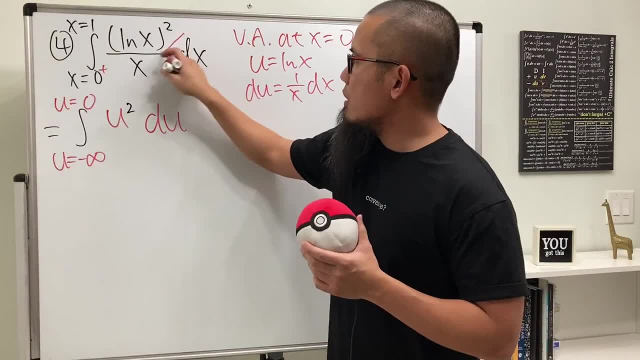 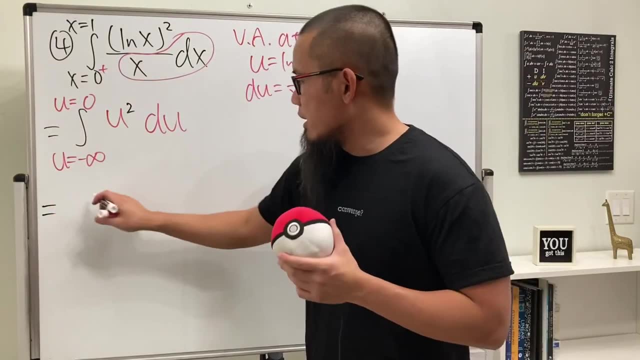 is precisely our du, so we can just, you know, pair them up and let's say: that's the du, so it's not so bad, let's just integrate. and this is what happens, right? let's see this right here: gives us one third u to the third power, and then we'll just have to plug. 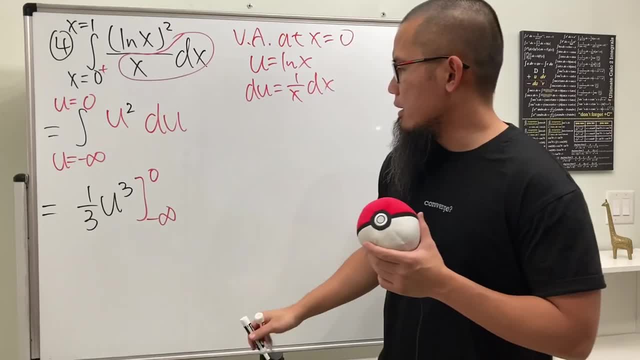 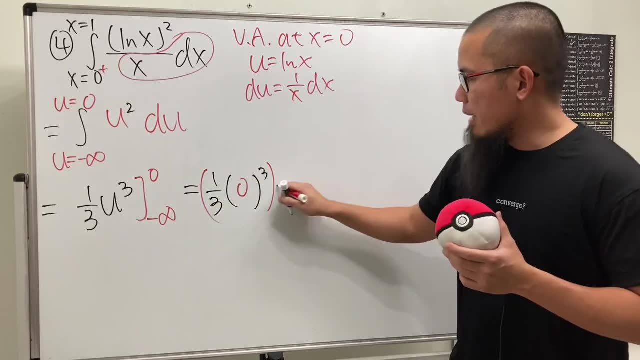 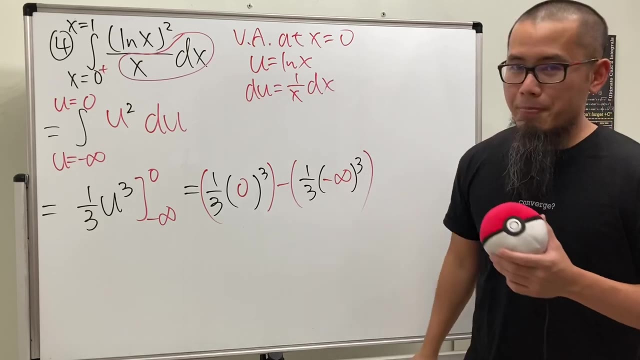 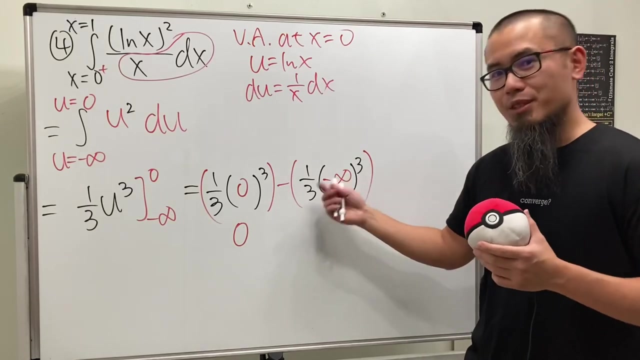 in, plug in, plug in right, and let's see, we will get one third and then zero third power, and then minus one third and then negative infinity third power. yeah, check this out, this is zero negative infinity. two third power's negative infinity times one third- still negative infinity. 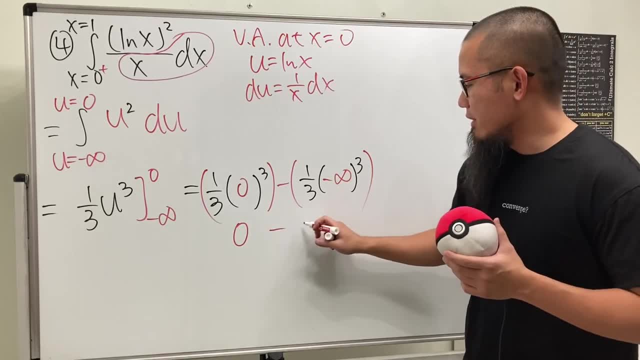 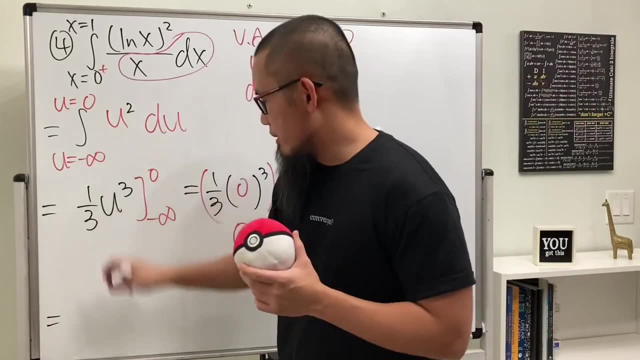 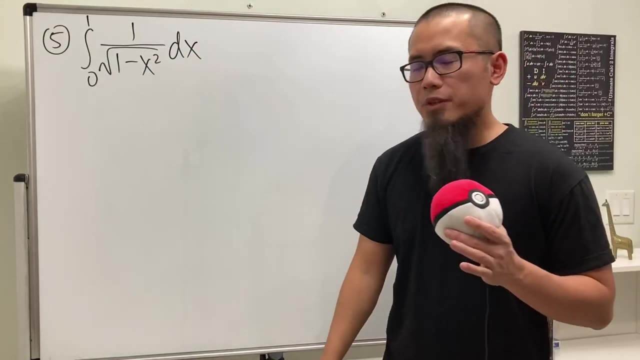 times negative, we get. well, i'll just say, like this, negative and negative infinity, yeah, but anyway, this right here is clearly infinity, so this right here diverges to infinity, just like that. all right. number five: we are integrating from zero to one of one over square root of one minus x square. where is the vertical house of the program of elimination? okay, we should be able to integrate this from 0 to 1, or from 1 over square root of 1 minus x square. 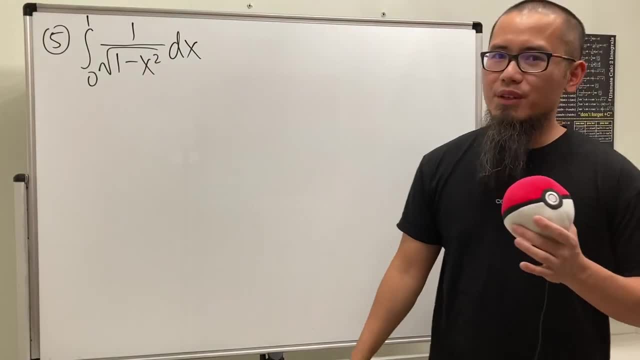 we should be able to integrate this from 0 to 1 of 1 over square. root of 1 minus x square. where is the vertical house of the problem here? this is minus infinity. we also can root of 1 minus x square. where is the vertical hospital? at 1 right. otherwise you see that on. 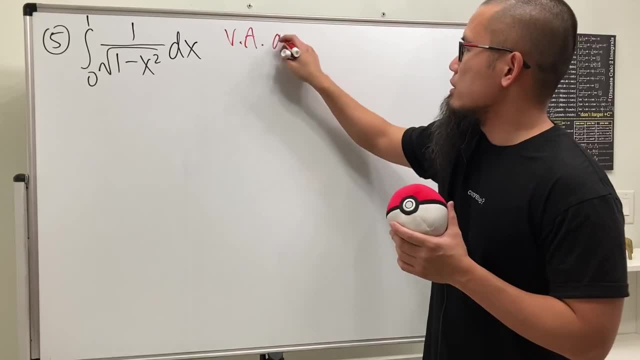 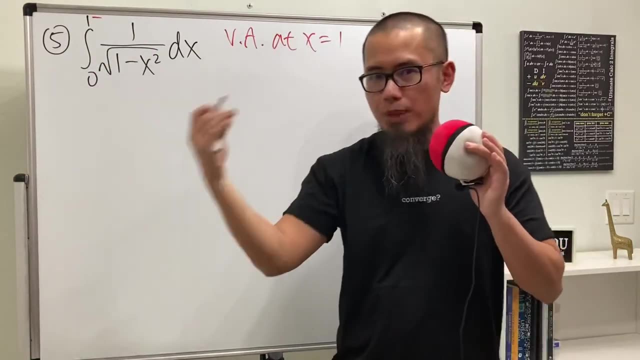 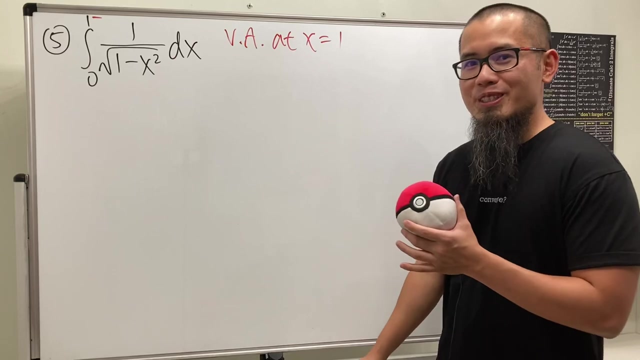 the bottom, we get 0. so let me just indicate that, real quick, vertical hospital at x equals 1 and 10 equal to. here we are doing 0 to 1 minus right, so we are approaching 1 from the left hand side. what should we do to integrate this, though? well, all we have to do is just know our derivative. 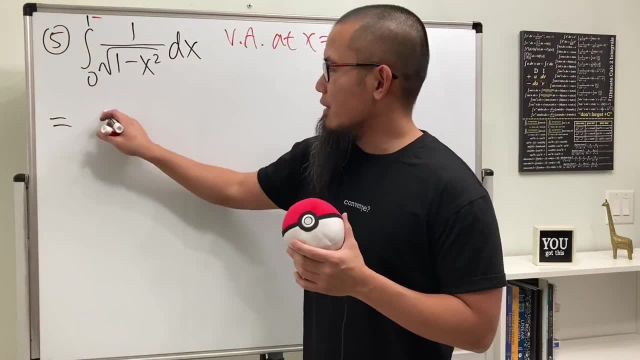 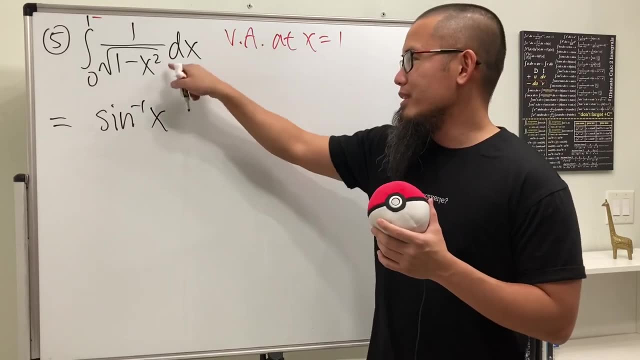 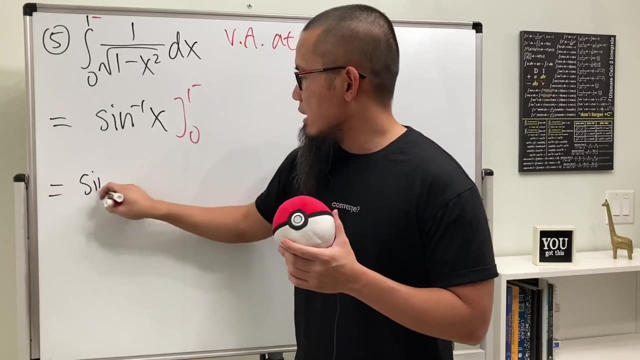 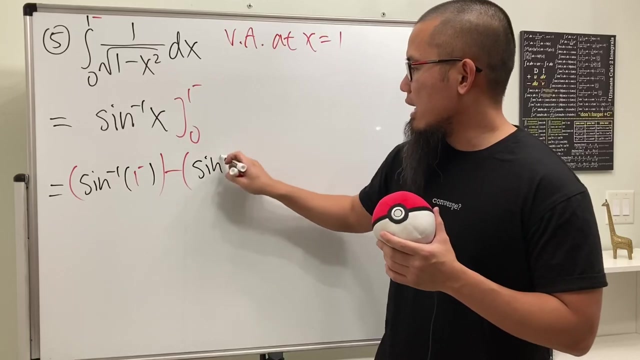 really well, because the derivative of inverse sine of x will give us 1 over square root of 1 minus x square. so integral of that is just this: all right, and then we go from 0 to 1 minus and plug in. plug in, we get inverse sine of 1 minus and then minus. plug in 0, we get sine and then. 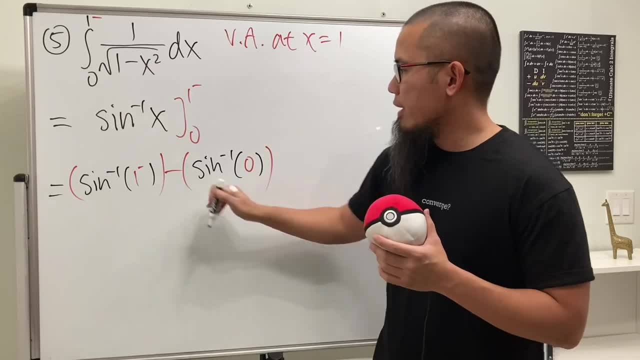 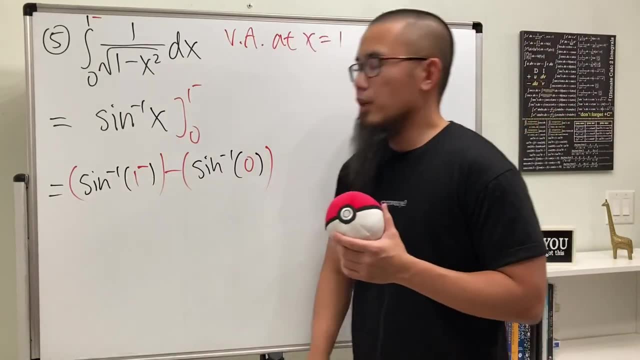 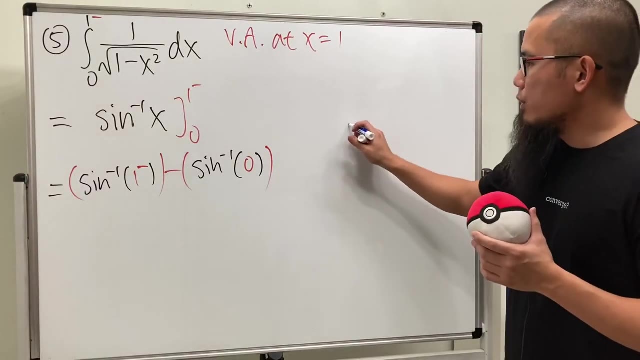 inverse and then 0 like this. okay, in fact, this right here is a good number to evaluate this. we'll just have to ask ourselves sine of what and go will give us 1. so let me just put that down right here for you guys. if you're looking at inverse, sine of 1 is equal to: i don't. 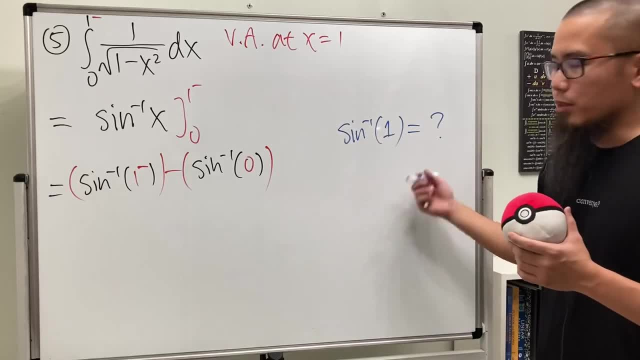 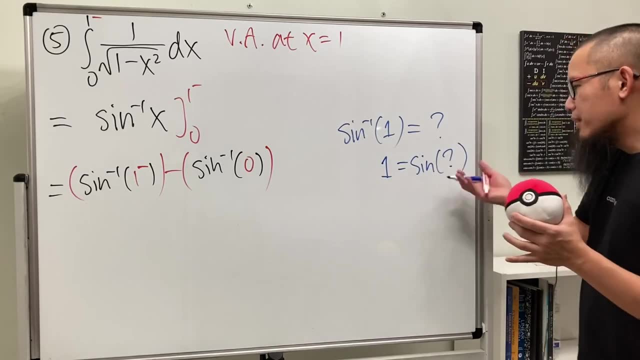 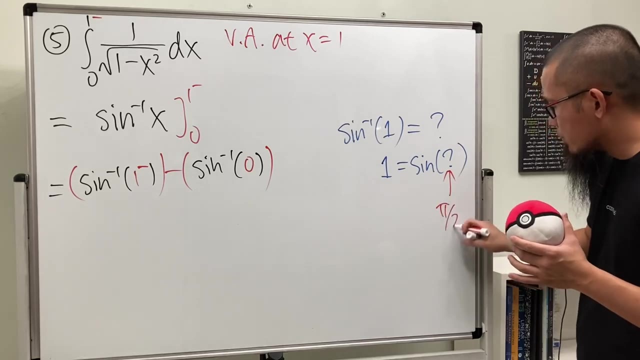 know, let's just say question mark. you can do the original sine on both sides, so you get: 1 is equal to sine of what, and in fact there are infinite many solutions to this right here, but you're going to pick like the first one, and that is pi over 2.. 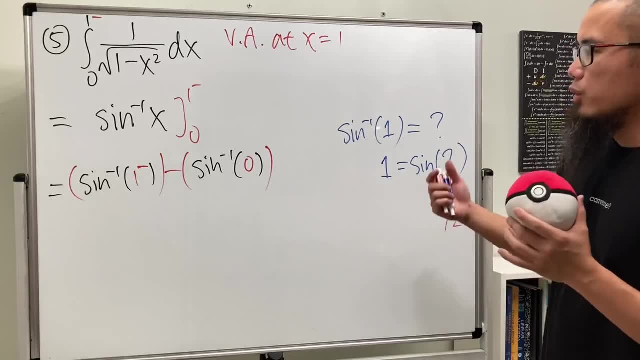 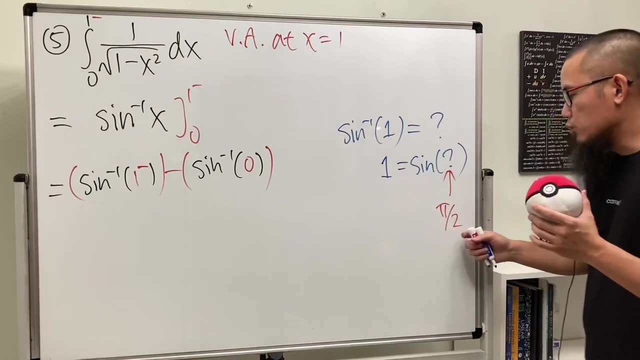 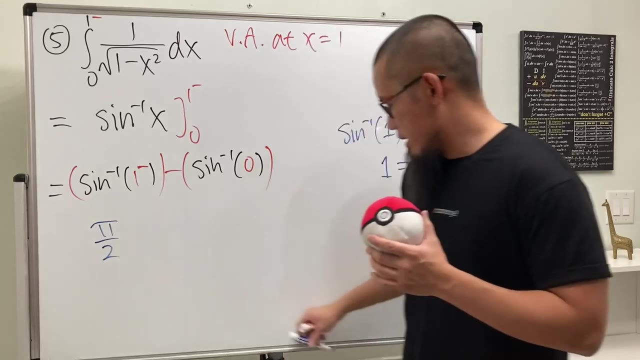 sine of power 2 gives you 1. so that's because the range of inverse sine function. it goes from negative power 2 to positive power 2. so this will be the only solution to the original. so this right here is really nice. we get pi over 2 and then 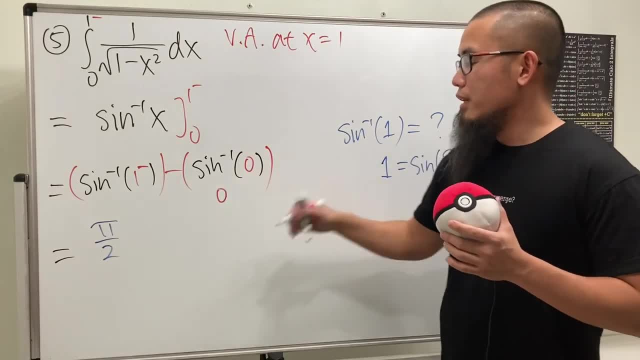 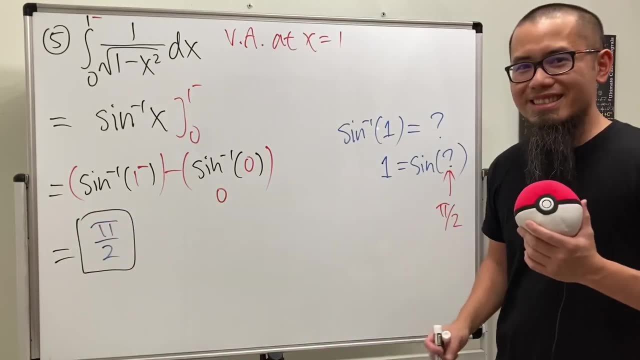 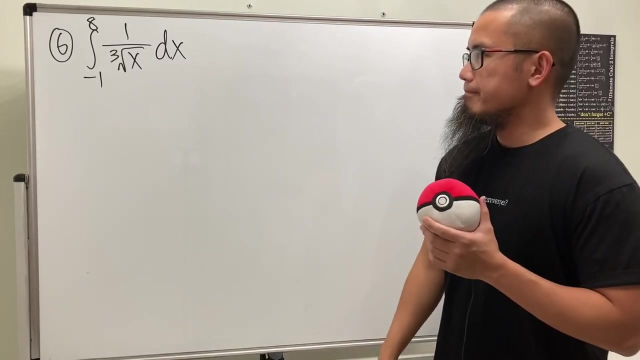 inverse sine of zero row is just equal to zero, because the original sign of zero: zero, so it's zero. so the answer is just power two. yeah, very nice, huh, okay, for number six, we have the integral going from negative one to eight of one over the cube. root of x. hmm, if you plug in negative one here, q. root of negative. 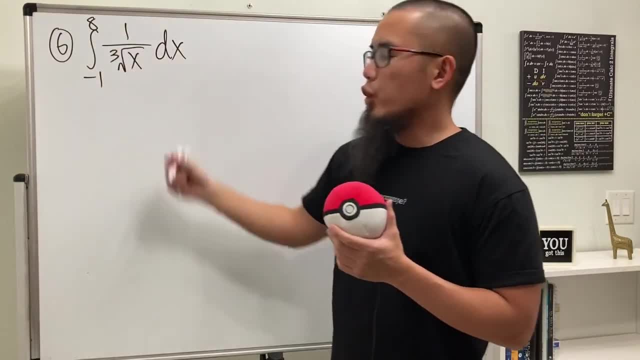 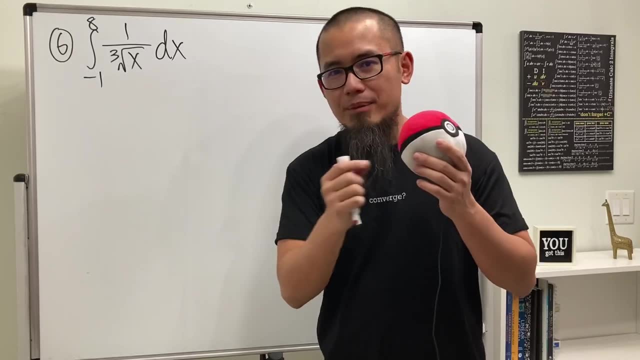 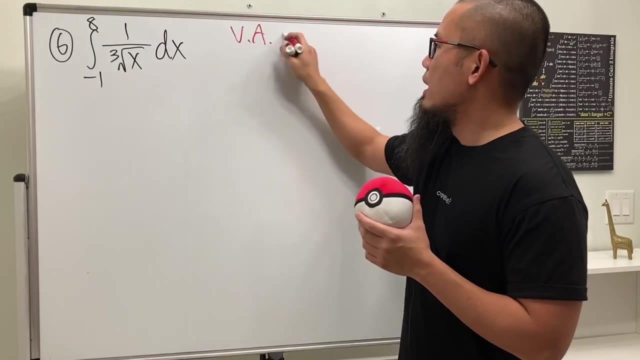 one is negative, one that works if you plug in eight in here. cube root of a is two. that also works. but remember we have to pay attention to: is there any number that will make the denominator zero right? and yes, we do this right here. it does have a vertical asset at x, equal zero if you look. 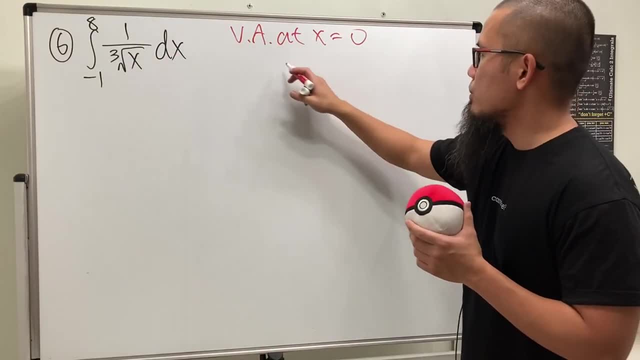 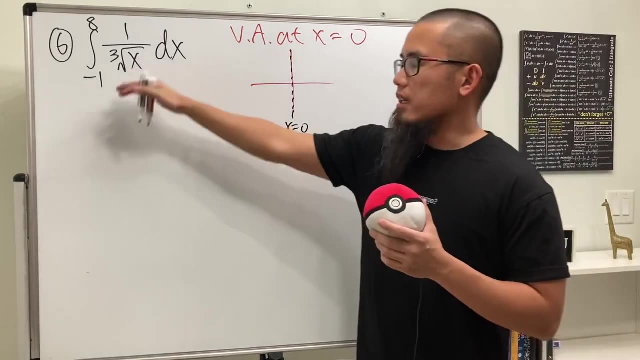 at the graph of this guy real quick. it looks something like this- i'm just going to put it down real quick like this: we have a vertical asset of s0 and when x is negative, you have a graph that goes down below like so: and then you have a vertical asset of x and you have a graph. 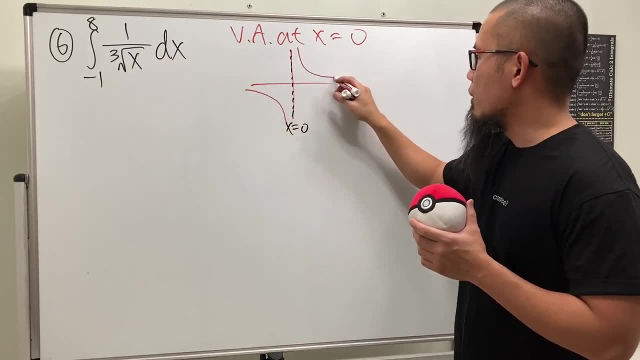 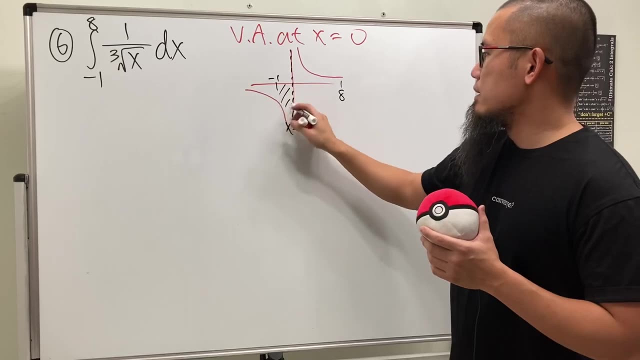 that goes down below, like so, and then you have a graph that goes down below, like so, and then you have x being positive. you have a graph that's above, like so, and we are going from negative one and then to eight, like this, and we're just going to find this and that the way to take care of this. 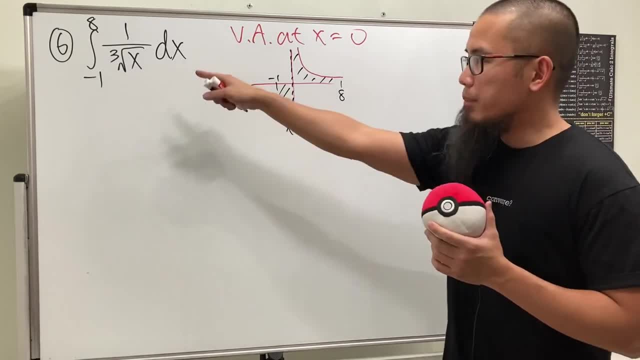 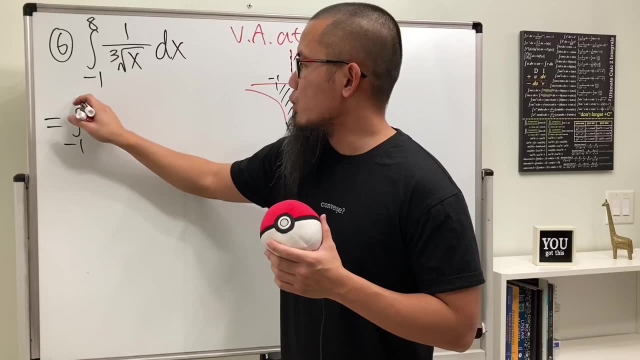 is that do not include zero. we have to break that part into two parts. so here we go. firstly, we are going to look at the integral going from negative 1 to 0. but we have to avoid 0, so we are going to 0, but we are going to avoid 0, so we are going to. 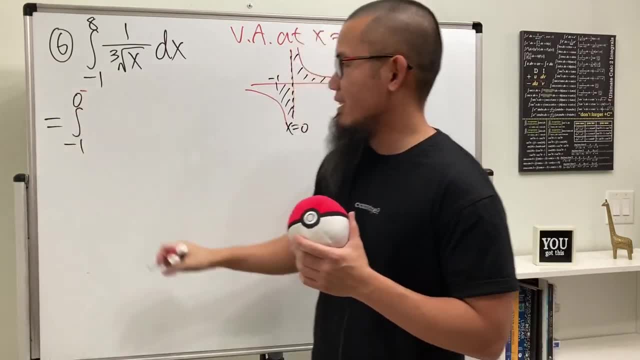 0. but we are going to, you know, do 0 minus right here, and then we have this guy which you know do 0 minus right here, and then we have this guy which you know do 0 minus right here, and then we have this guy, which i'm just going to write it as: 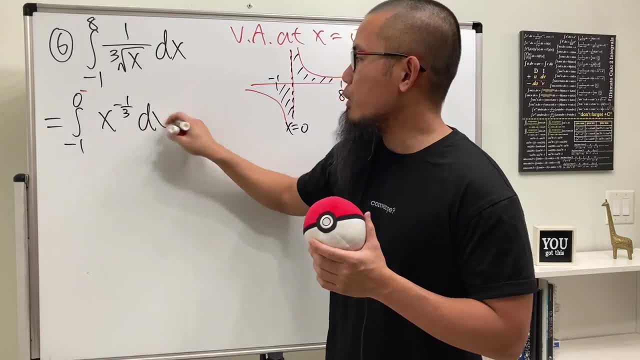 i'm just going to write it as i'm just going to write it as: x to the negative 1 third power, because we are x to the negative 1 third power, because we are x to the negative 1 third power, because we are about to integrate that. 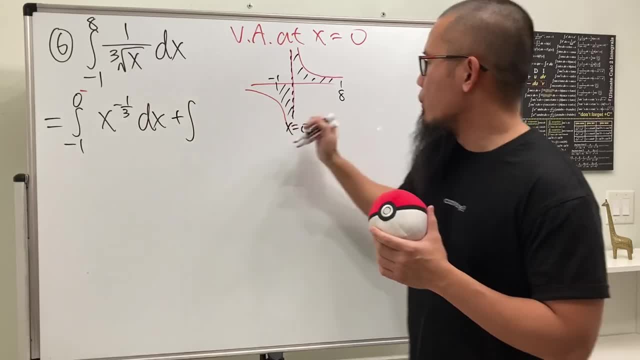 about to integrate that, about to integrate that, and then we are going to add, and then we are going to add, and then we are going to add: well, we have to, well, we have to well, we have to. this was zero minus. we have to pick it up. 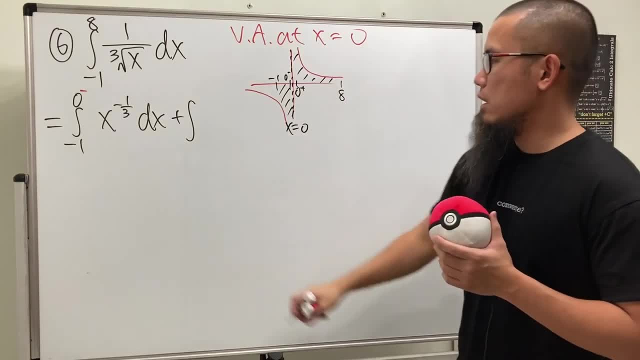 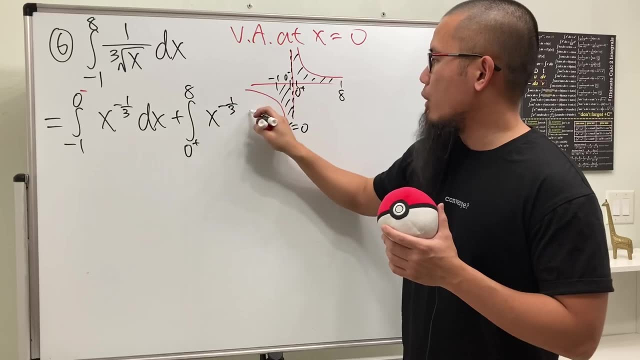 this was zero minus. we have to pick it up. but we cannot use exact zero, we use zero plus. so we go from zero plus up to eight, and then again we can write that down as x to the negative one third power. good, and now we can just take care. 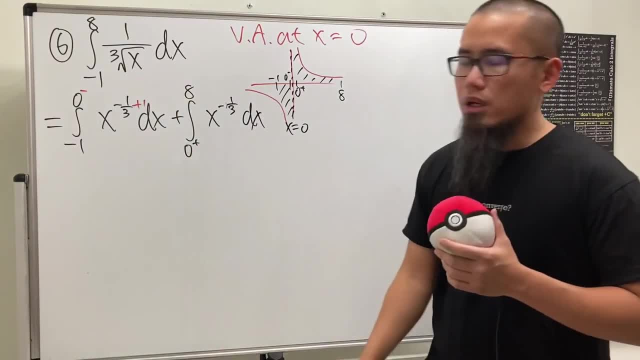 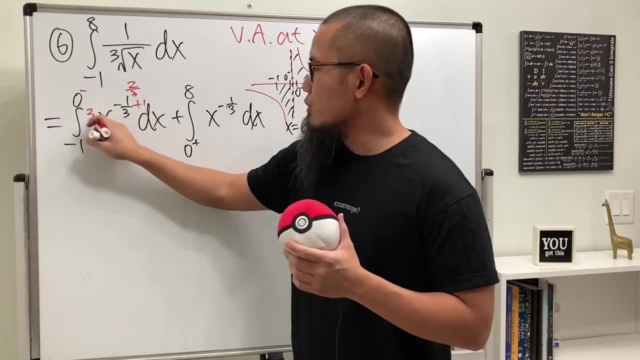 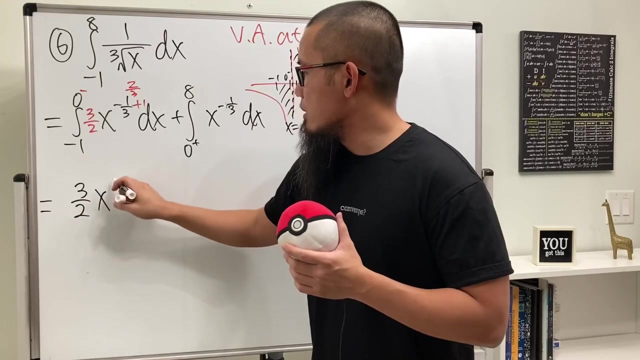 of each, every part. for this one, we add one to the power. negative one. third plus one is two third. yes, yeah, and then, divided by the new power, we get three over two. all right, so for the first one we get three over two, and then x to the two over three, and then we will have to plug in numbers. 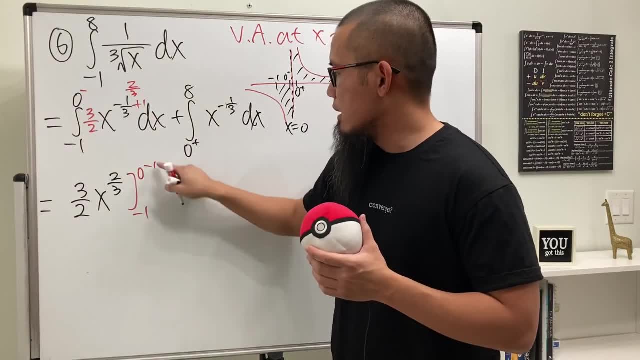 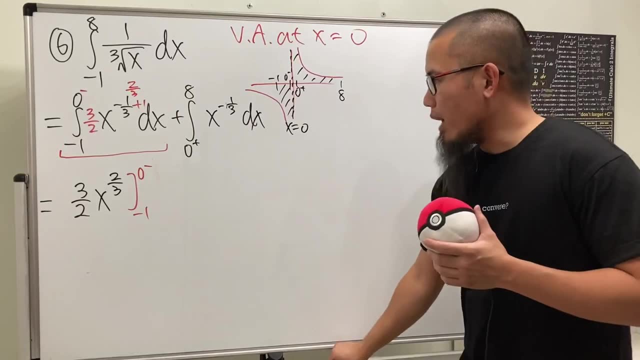 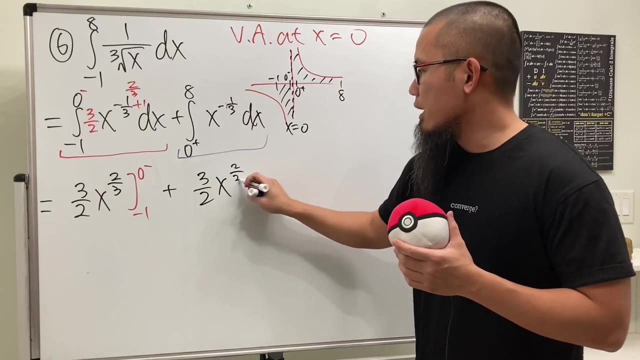 right, so plug in negative one and plug in zero minus. so that will be the first part, right here in red, i would say. and then for the second one, i will do this in blue: i'm going to add, well, 3 over 2 x to the 2 third, and then we will have to plug in 0 plus and then 8.. all right, 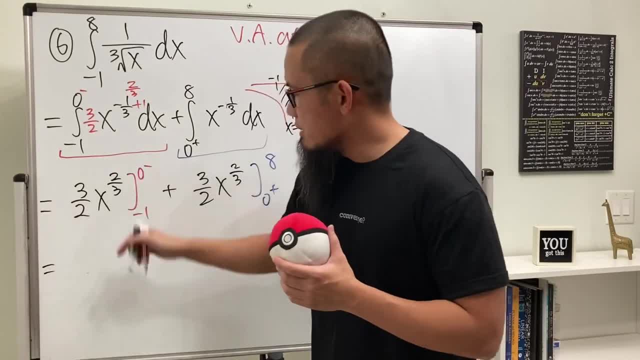 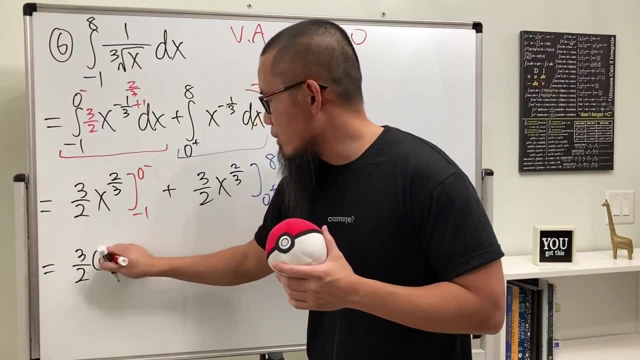 so so for this one, okay, let's just do the work, plugging 0 minus, which is just 0, because this guy is really nice. here we have 3 over, 2 times 0 minus, and then 2 over 3. this is the first one. 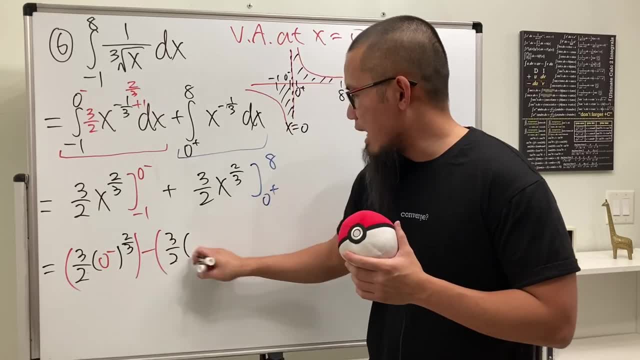 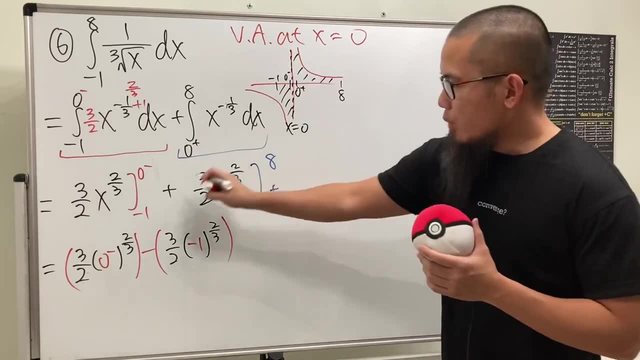 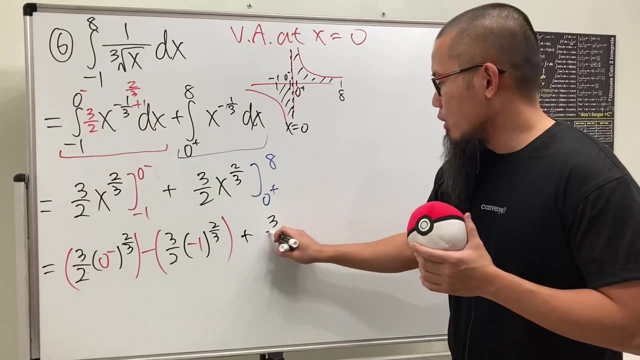 and the minus parentheses: 3 over 2 times negative 1, and then to the 2 over 3. all right, good, and then we are going to add this one i'm going to do in blue: in terms of plugging the number, we get 3 over 2, and then 8, and then 2 over 3, and then plugging the. 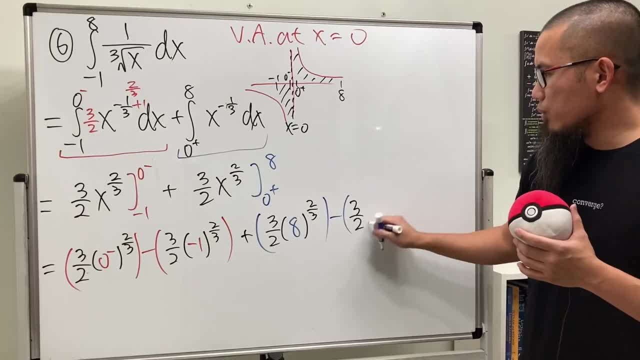 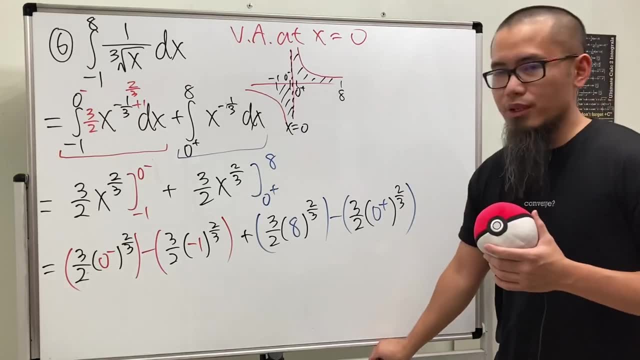 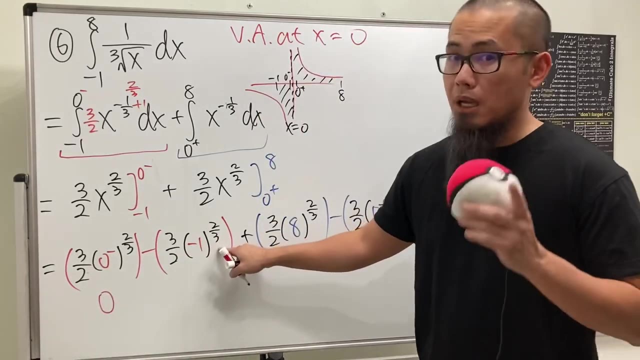 the zero plus, we get minus parentheses, 3 over 2 and then 0 plus and then 2 over 3.. yeah, so far, so good. okay, check this out, this is just zero, so that's good. and then this is going to give us positive 1. right, this is going to give us positive 1.. so we will have 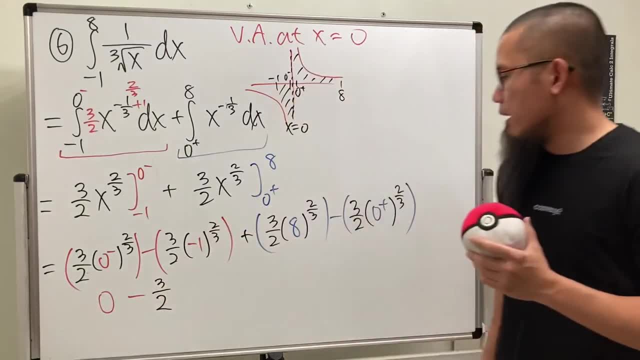 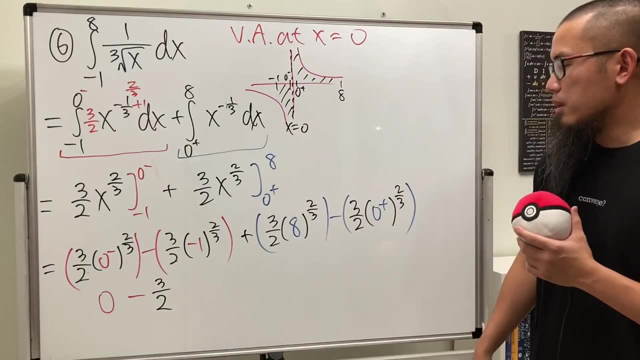 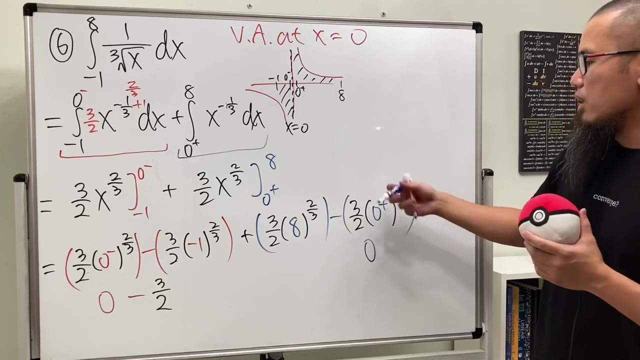 have to minus 3 over 2. all right, so this right here actually converges, because when we have the triple number here it does give us a finite value. but then we just have to do the fractions. this part right here is just 0 as well, but let's compute 8 to the 2 over 3, and let me just remind: 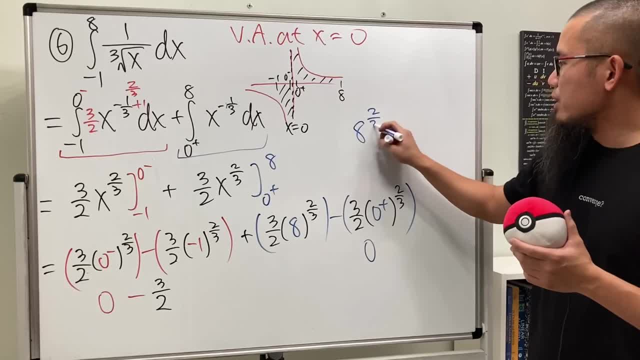 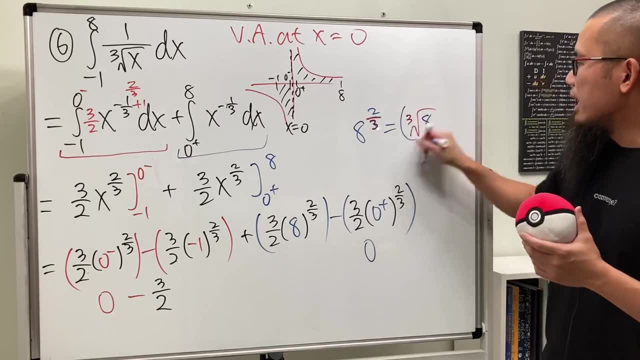 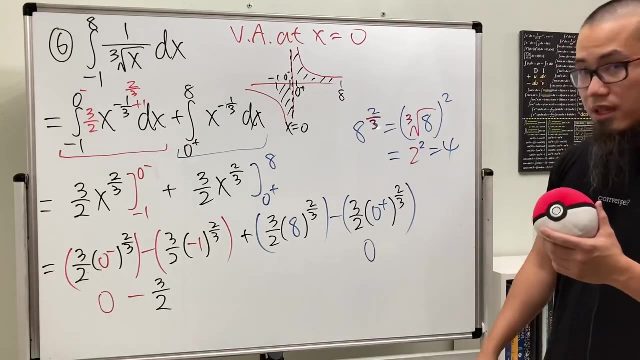 you guys, the google algebra, days 8 to the 2 over 3. what you do is you look at this as the cube root and you do that, first cube root of 8, and then you do the square on the outside. cube root of 8 is 2 and you square that. so the answer for this is 4. yeah, okay, so this right here. 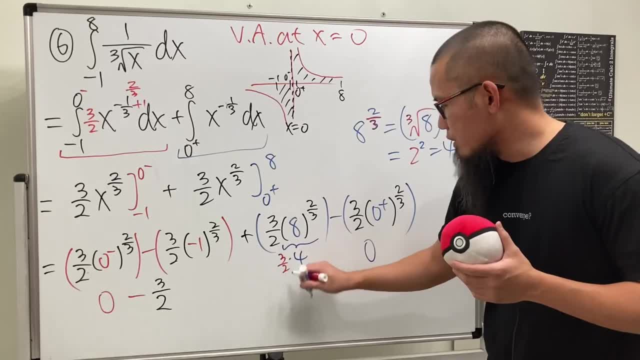 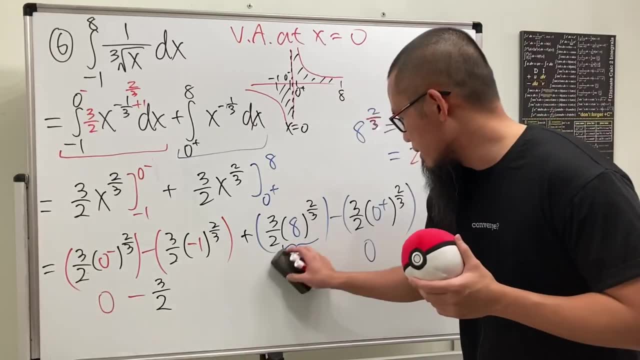 is 4, but you multiply by 3 over 2, so without a fraction you will get 6. so right here we just have to add 6. so perhaps just keep the same color: 3 over 2. so we are just going to add 6. 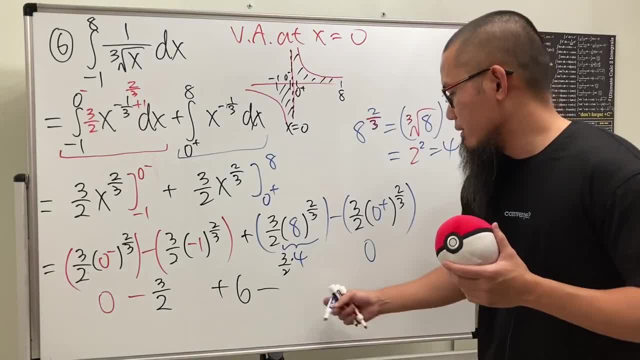 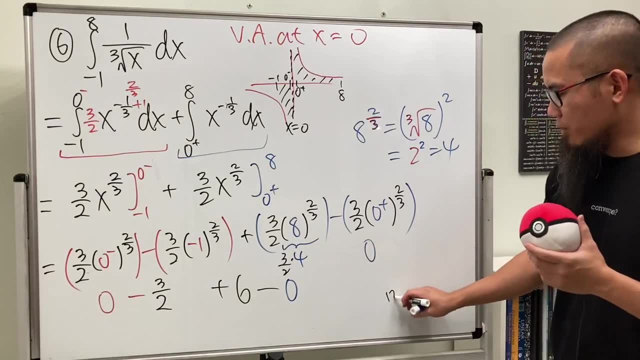 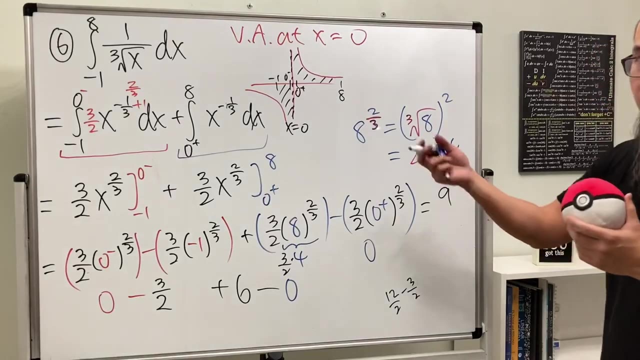 and then minus 0, and this has a lot of fractions, all right. so finally just do 6 minus that, so it's 12 over 2 minus 3 over 2, which is 9 over 2. so all together, this right here converges to 9 over 2. i. 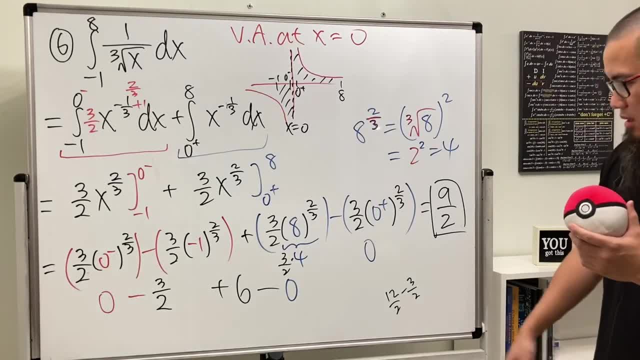 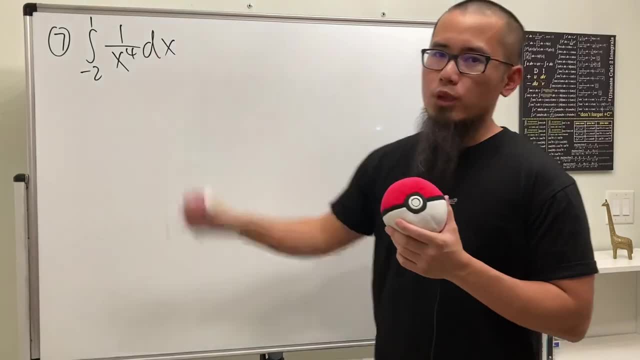 hope i didn't add the fractions wrong. we'll subtract the fractions wrong. yeah, so that's it for number seven. we have the integral going from negative two to one of one, over x to the fourth power. this is similar to what we did earlier, because the vertical 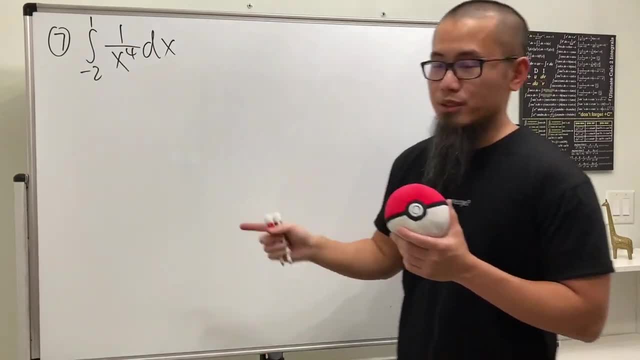 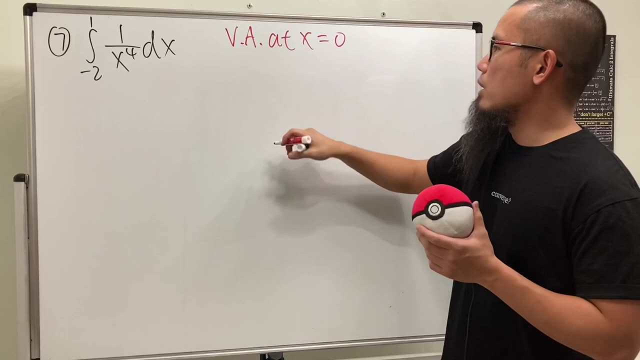 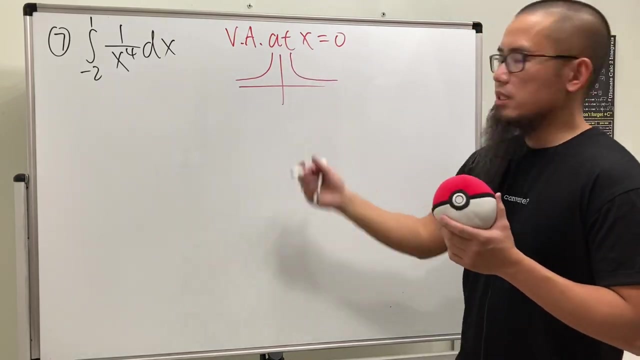 isotope is not at the end point, it's actually at zero, it's just somewhere right in between. so let's just indicate that vertical isotope at x equals zero. and if you want to see the graph for one over x to the fourth power, you will look something like this: like a volcano, very similar. 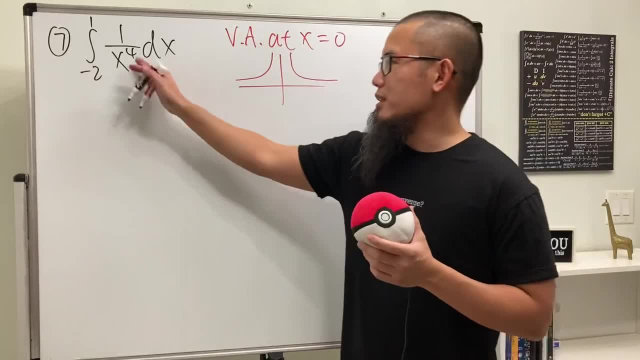 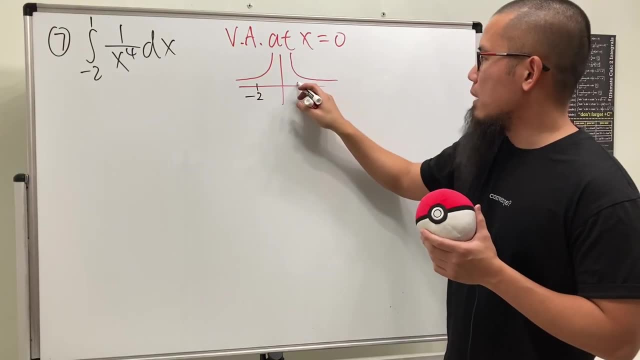 to the example that we did in class. in fact, i just changed the second power to a fourth power. right, by the way, let's just go ahead and do all this. we go from negative two to positive one, so we are taking a look at here and also here. of course, we do not want to have exact zero. 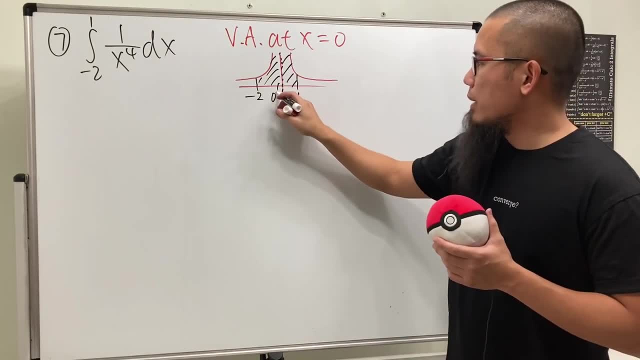 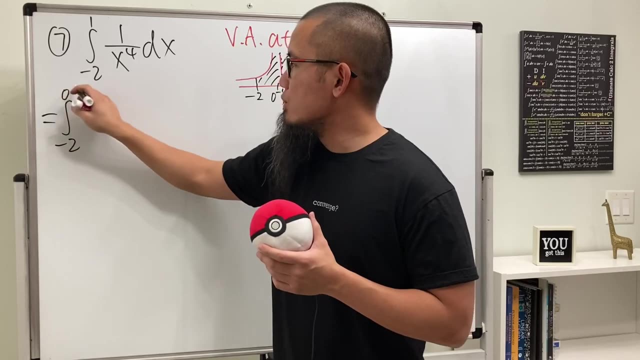 so what we do is break it apart, right? so look at zero minus and also zero plus. all right. so for this one, we are going to get the integral going from negative two to zero minus first, and then look at this as x to the negative fourth power, dx, and then we are going to 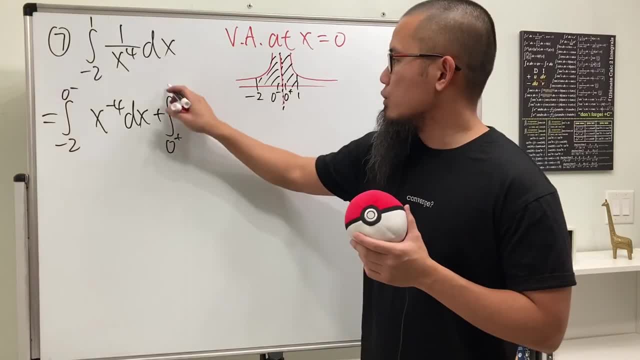 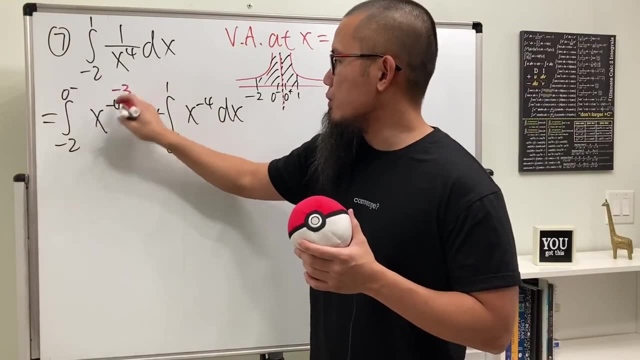 add. and then we are going to add x to the negative fourth power, dx. and then we are going to add- we are going to pick that from 0 plus to 1, and then x to the negative 4, dx. now integrate this, add 1 to the power which is negative, 3 divided by the new power, and we get that and we get negative. 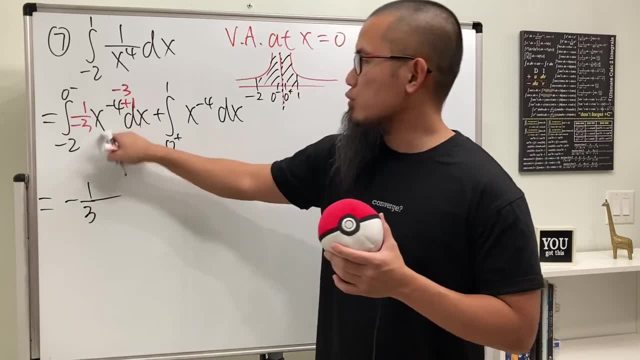 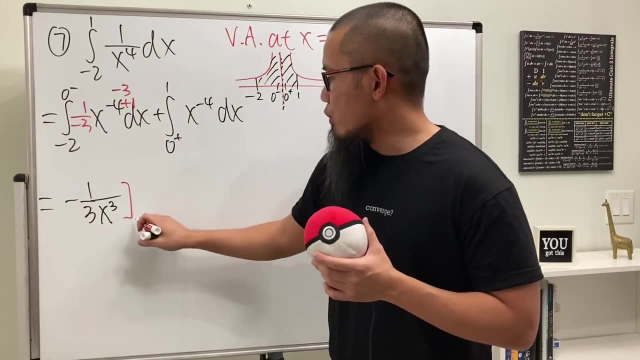 1 over 3, and then perhaps let's just put the x to a negative 3 power down here and becomes x to the third power. okay, and then we will have to go from negative 2 to 0 minus, and then we are going to add. 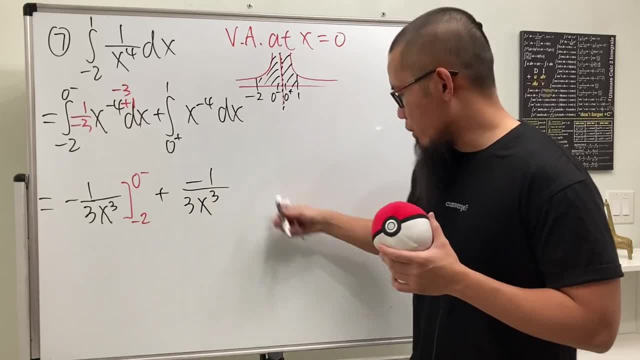 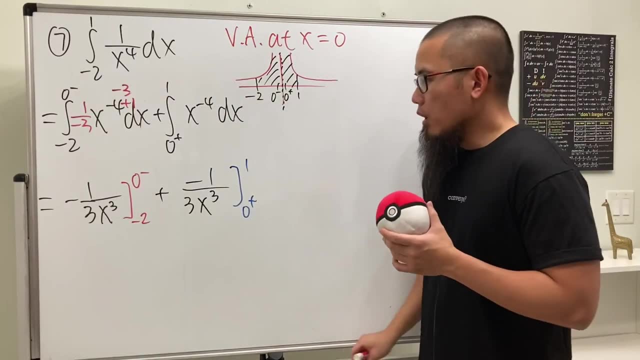 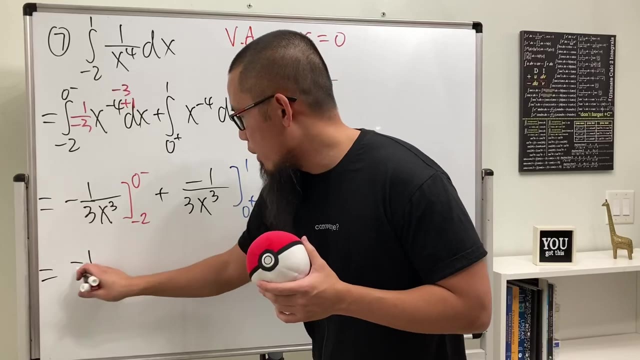 which is negative 1 over 3x to the third power, but plug in 0 plus and 1, yeah, all right. so let's just go ahead and do the plug-in for this. plug-in 0 minus first and we are getting negative 1 over 3. 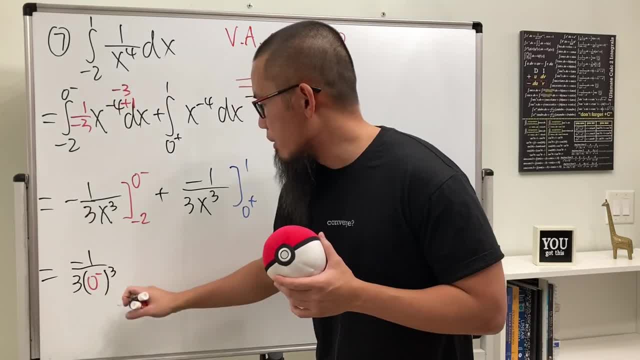 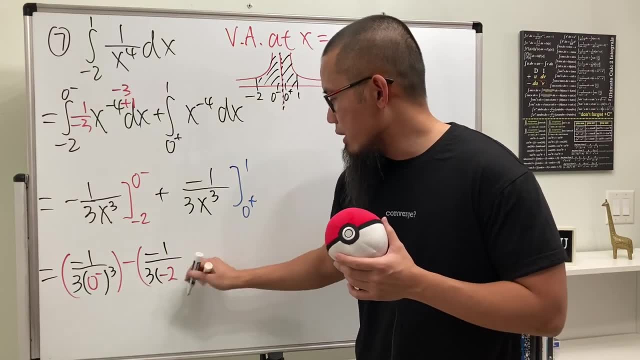 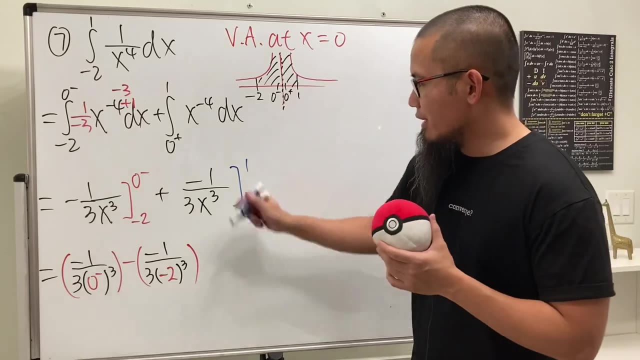 times 0 minus. and then to the third power. that's the first term minus the second term: negative 1 over 3 times negative 2.. and then to the third power. for this, of course, i'll plug in the numbers in blue. we get well first. 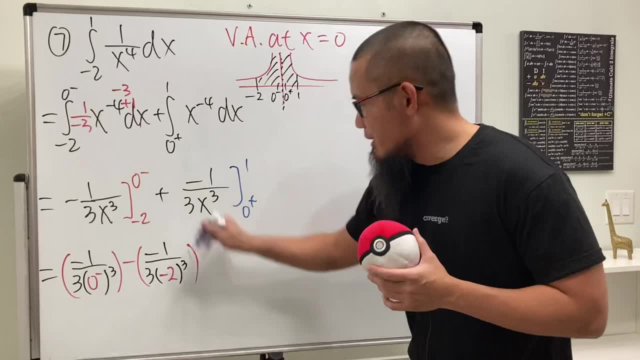 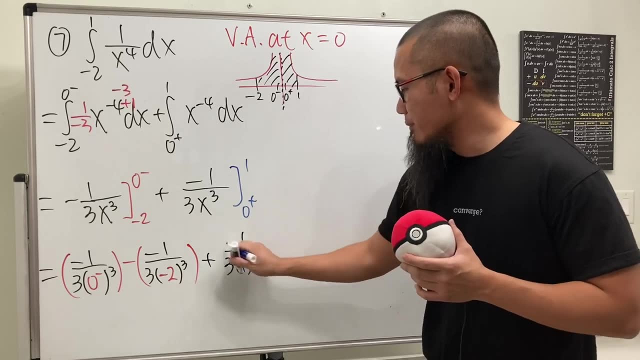 we put down plus wrong color. we first put down the plus and then we plug in 1, so we have negative 1 over 3 times. 1 to the third power and the minus plug in 0, minus, so we get negative 1 over 3 times. 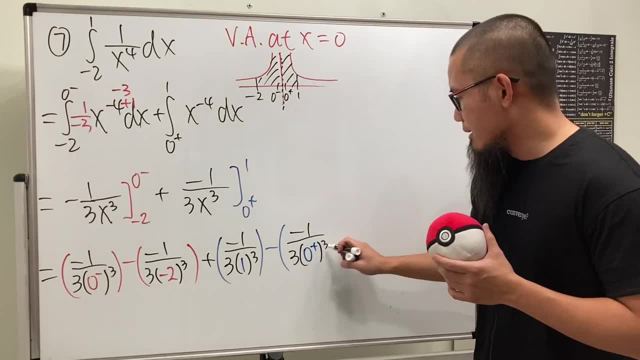 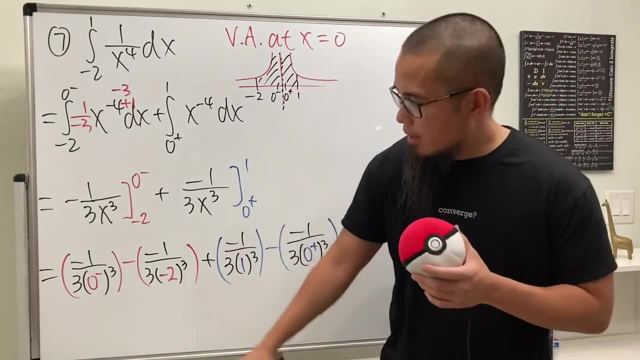 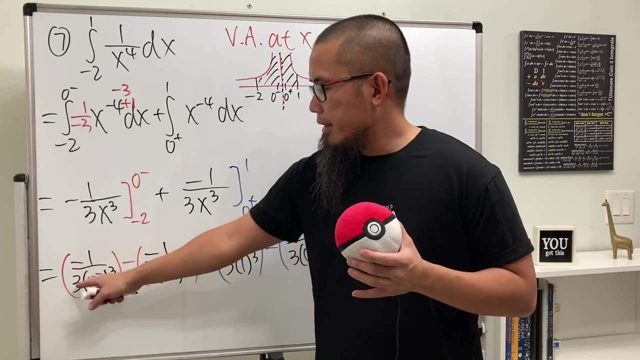 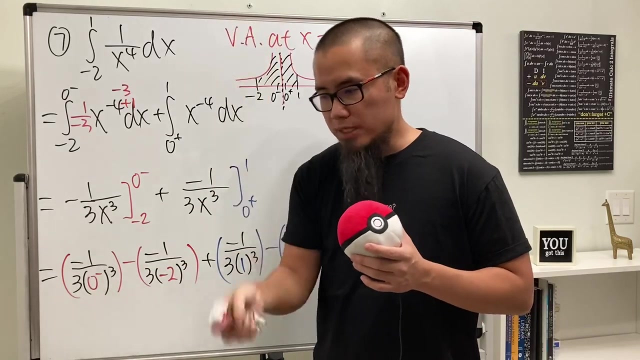 sorry, 0 plus. yeah, okay, cool, very cool? not really, because you see that this right here, 0 minus to a third power, that will still give you a negative right. so it's technically still 0 minus and then multiplied by three is still 0 minus. and then on the top here we have negative one divided by 0 minus. 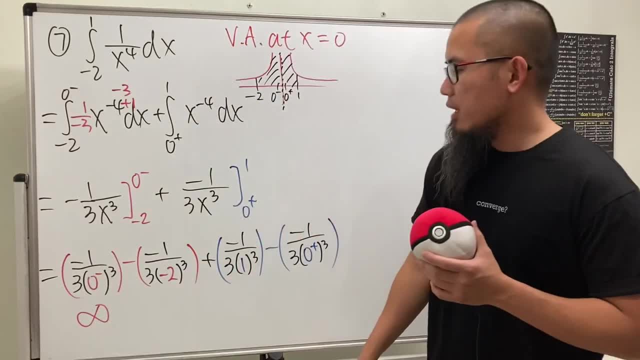 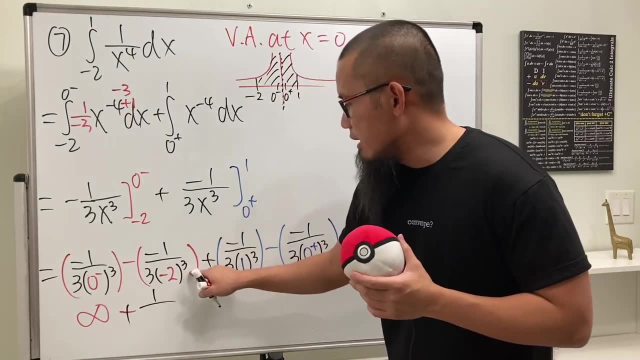 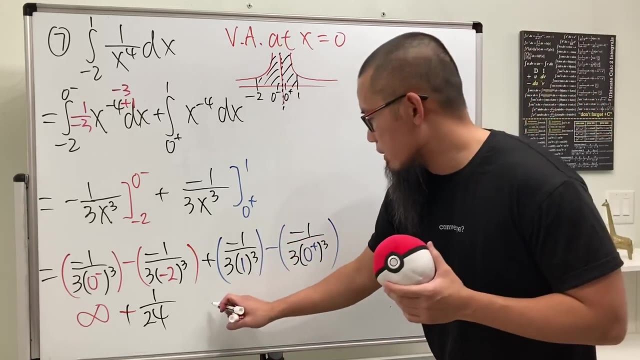 so altogether this will give us positive infinity. and this number we don't really care, but i will still compute it real fast. this is one over negative 8, right? that's how i make this positive. and then 8 times 3 is 24, and then for this we are. 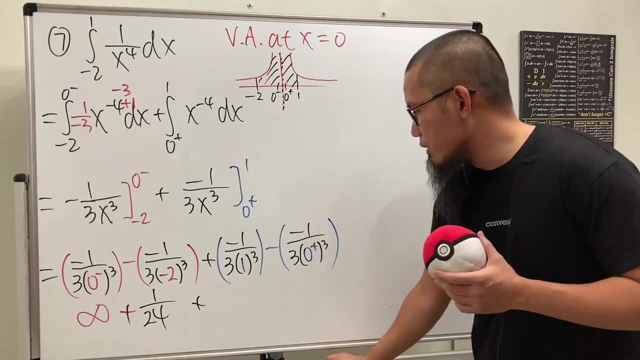 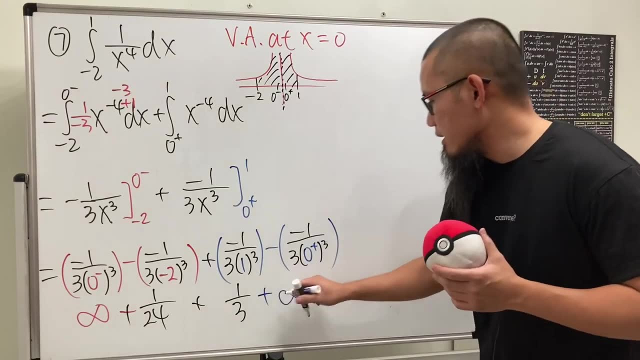 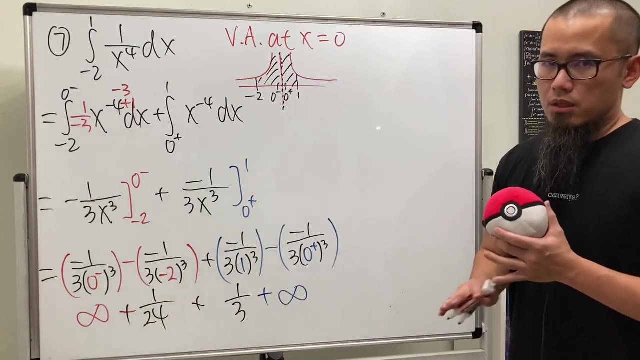 going to add. this is just 1 over 3, so that's good. and then minus minus becomes plus and then we have infinity, like. so, as you can see, we have infinity and plus infinity. so this right here is not debatable, it's just go ahead. positive infinity, and you can look at it from the graph right here. 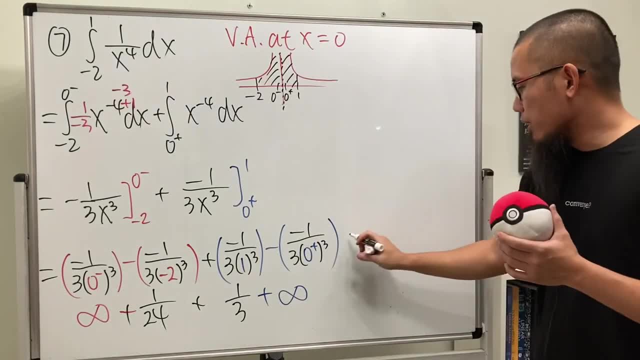 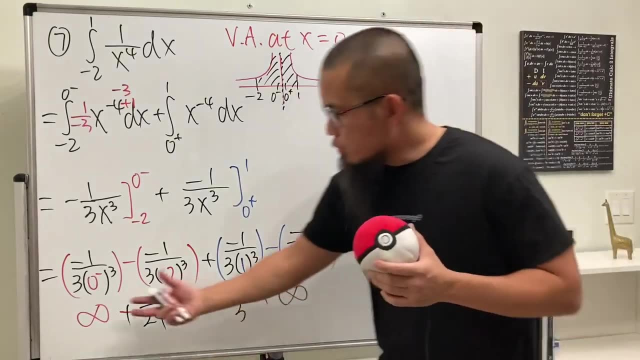 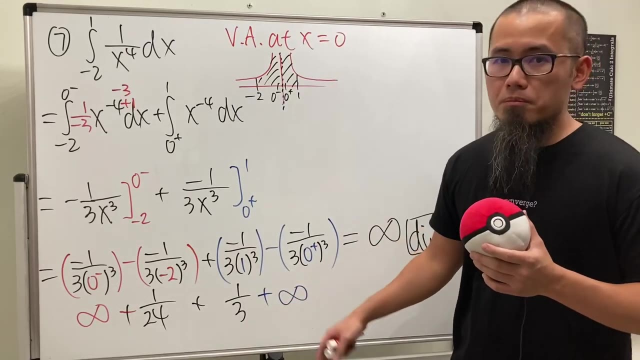 as well right infinity. so this right here diverges to positive infinity. what if this right here gives us gives us a red infinity and it's positive, and this right here gives us a negative, blue infinity? in that case we cannot do a thing. and the idea is, whenever we break down an improper integral, 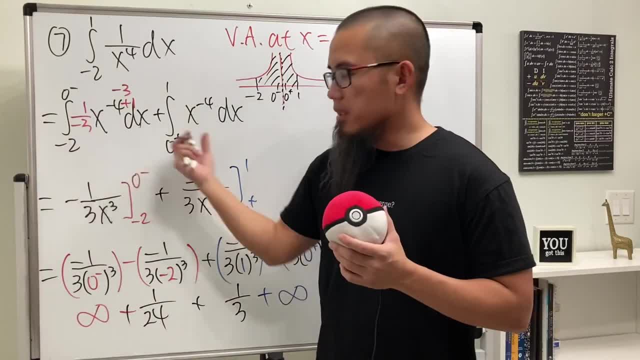 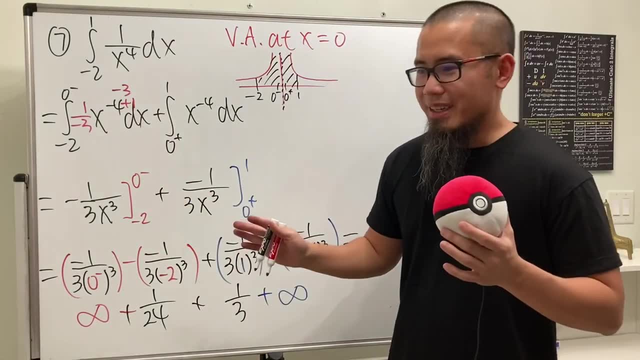 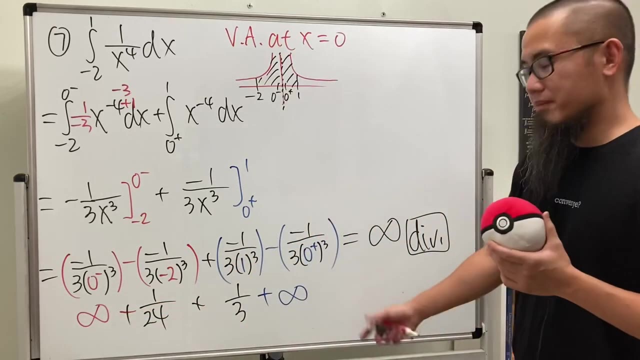 into two pieces. as long as one piece or one part of them diverges, the whole thing diverges. end of arguments. end of the work. yeah, but this right here, don't even worry, because that thing's really clear. that's it. you know, you, i'm going to ask you guys a question that has to do with partial fractions. this is the one. 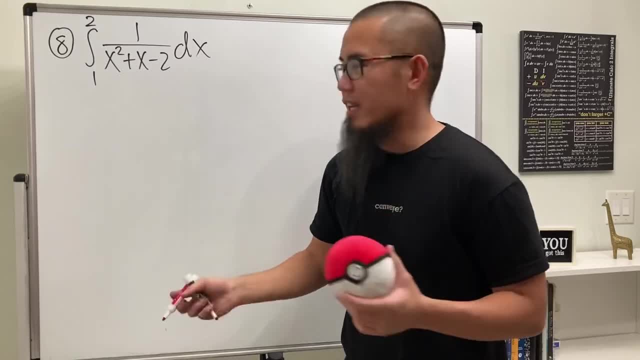 if you look at the bottom here, can we factor it? yes, so let's go ahead and factor it. we get x minus 1 times x plus 2, and then we get x minus 1 times x plus 2, and then we get x minus 1 times x plus 2. 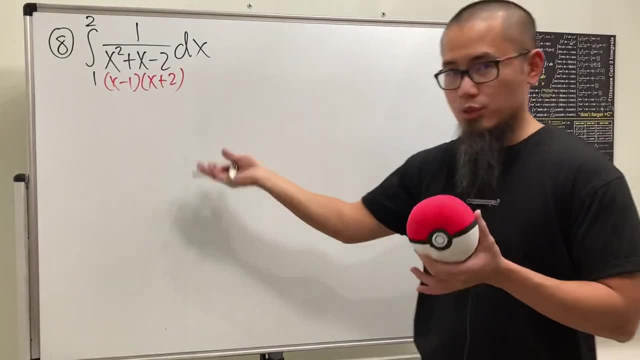 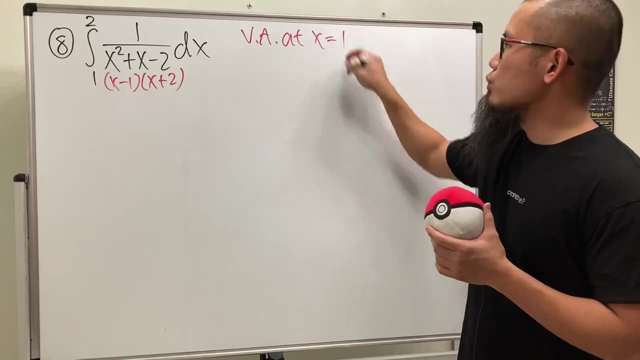 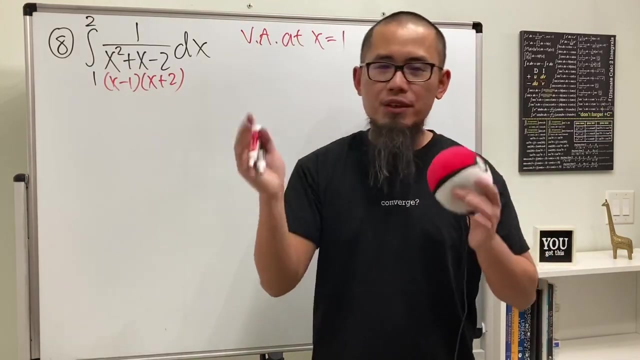 and you see that when x is 1, we get a zero on the bottom right. 1 over 0, we get that vertical acetope. so let's go ahead and indicate that vertical acetope and x equals 1.. at 2 is okay. sometimes if we have like both ends, gives us vertical no hope. in that case we still have. 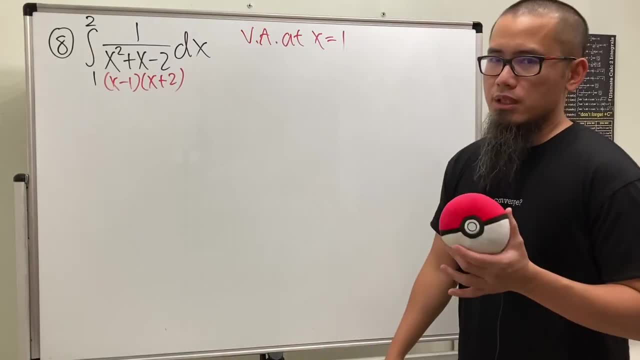 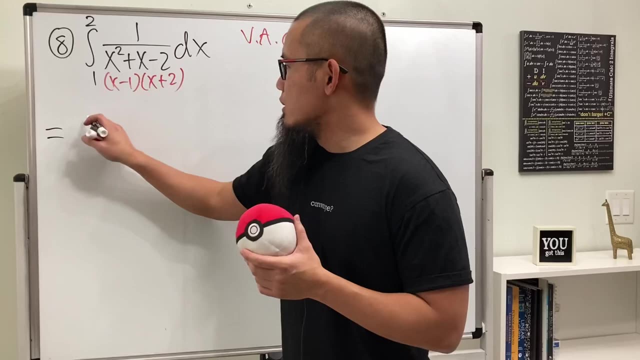 to break down into two pieces, but usually i won't ask you guys those kind of equations. i will test. by the way, partial fractions in action go from 1 to 2 and this one, technically, is 1 plus. so just keep that in mind, keep that in mind. 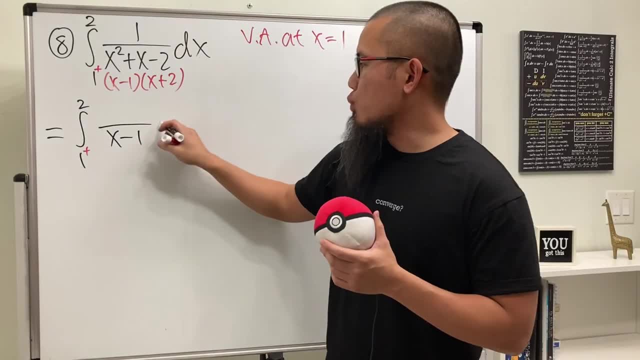 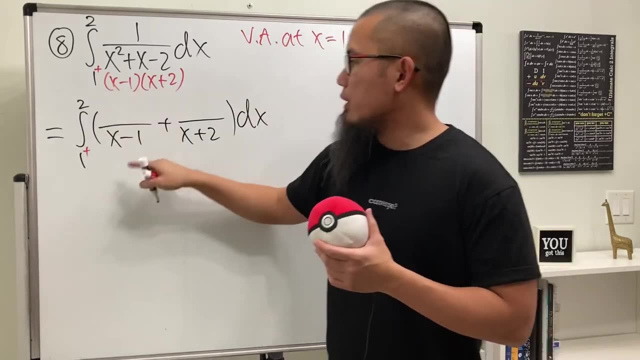 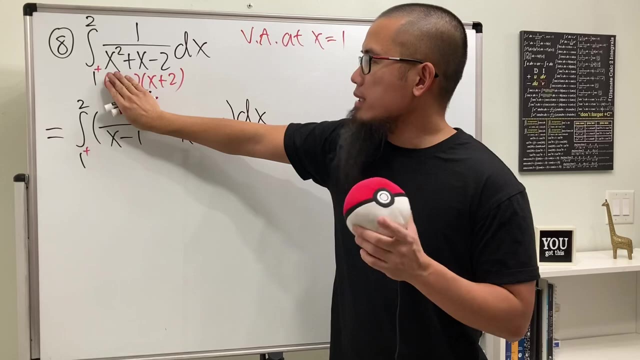 for the first fraction, we will have some number over x minus 1, and then for the second fraction, we will have some number over x plus 2.. good, all right, to figure this out, we go back to the original and cover this, and we will have to ask ourselves: what do we need to plug in right here? 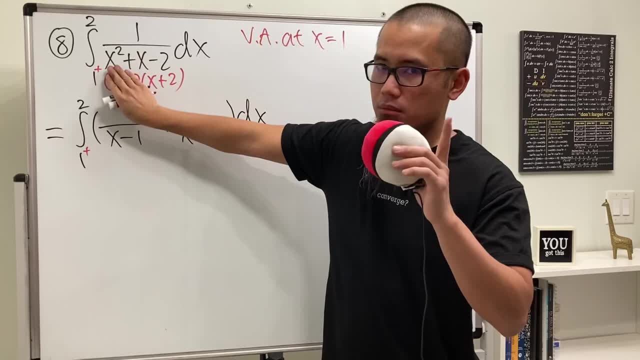 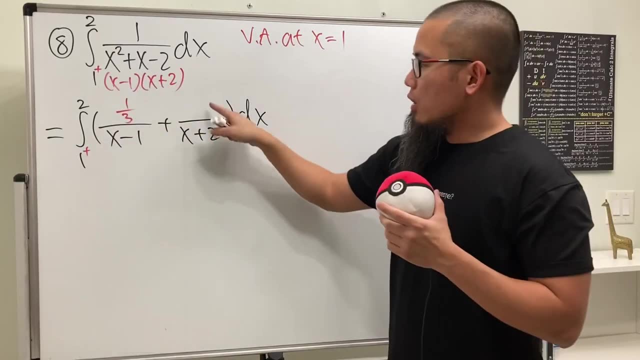 to make x minus 1 equal 0 and the answer is 1, and we are going to put a 1 in here: 1 over 1 plus 2, which is just one third. good, well, to figure this out, we go back to the original and couple this up. 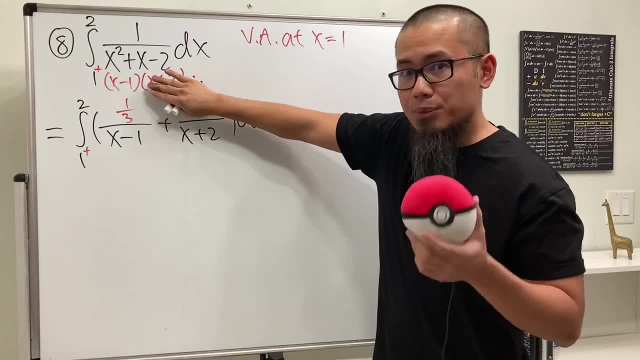 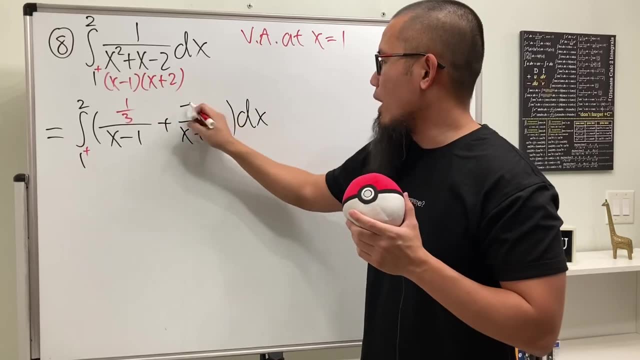 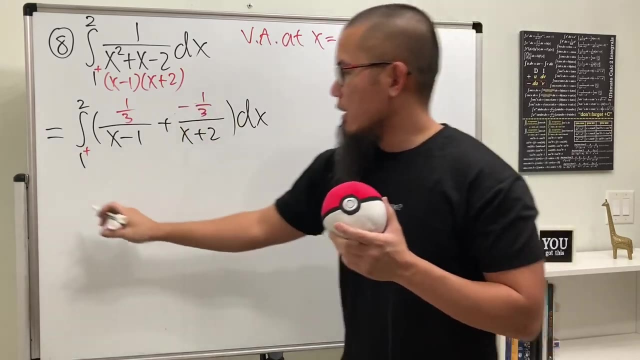 and how can we make x plus two zero? x has to be negative two and we put it here and we get 1 over negative two minus one, which is negative one third. perfect. so now we can just go ahead and ink, integrate for the first one, we'll just have one third, and then ln and we don't need to have 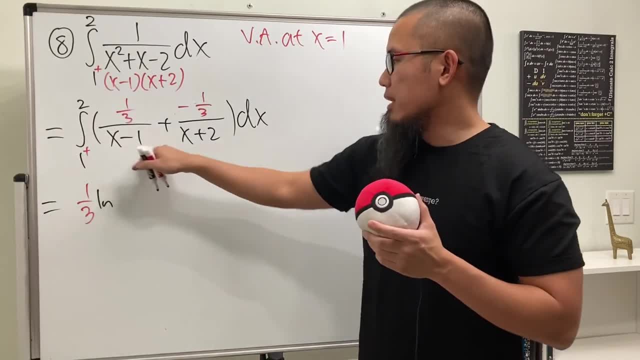 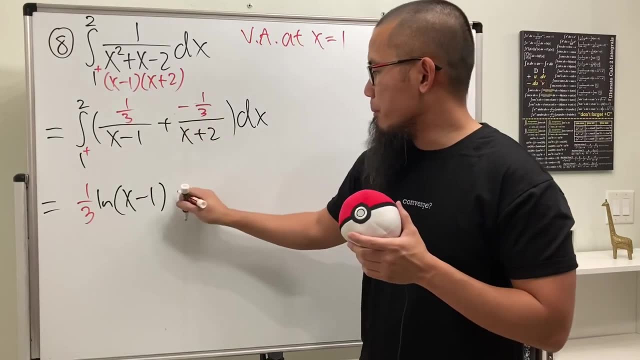 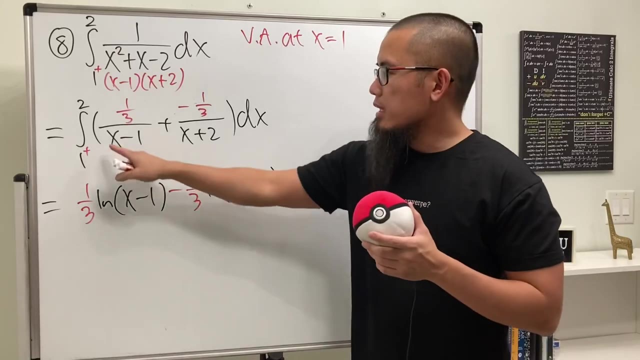 absolute value, because on this interval the x minus 1, x plus 2 will be positive. so don't worry. so let me just put on parentheses: x minus 1, and then we are going to minus one third ln, parentheses x plus 2, and again you see that this is the integration and the coefficient of x is: 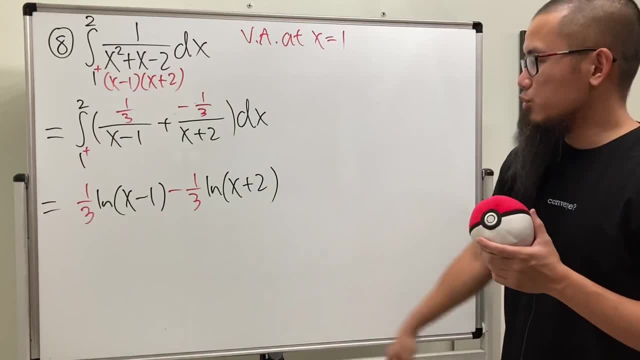 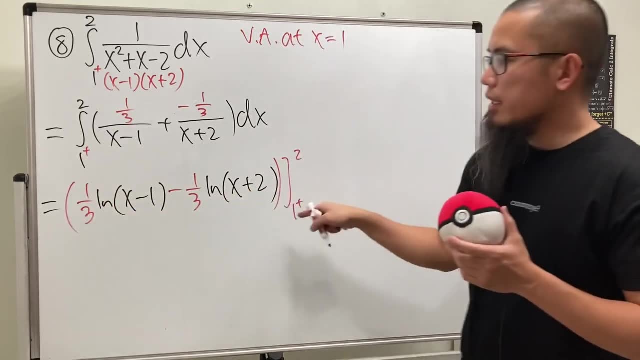 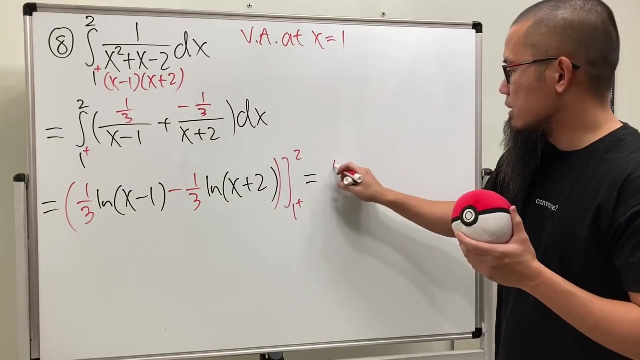 just one so we do not have to divide anything else. so that's really nice. and before we plug in the numbers, perhaps it's a good idea to combine the natural logs together first, and when we do that we will get one third first. so let's put that down and then ln this will go to the top. 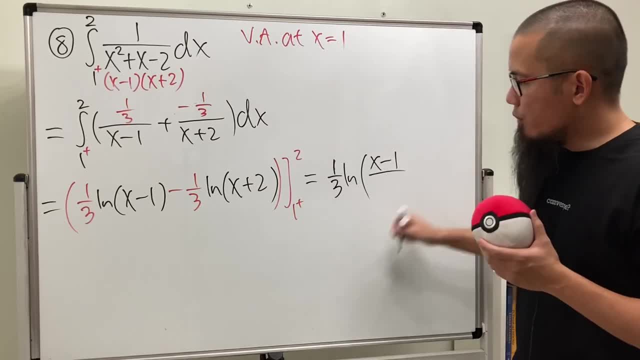 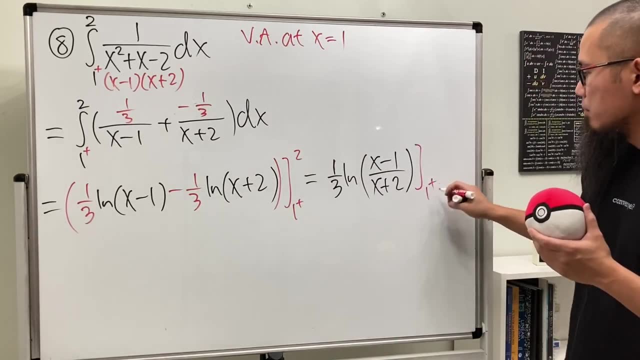 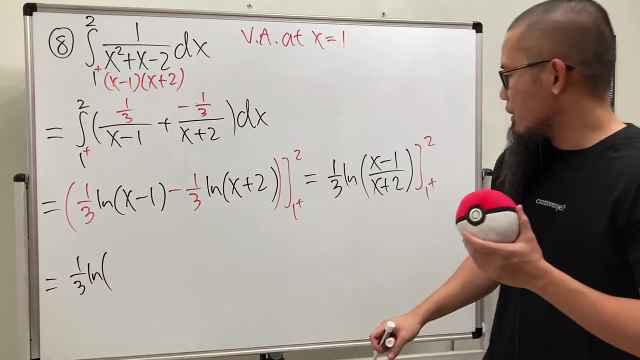 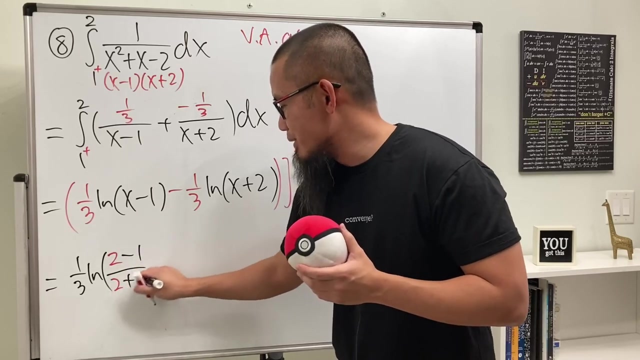 because it has positive right here over, this right here will be on the bottom because it has the negative right, you cool. and then we plug in. plug in, all right, plugging two, we get the following: we get one third ln parentheses- two minus one over two plus one. oh sorry, two minus one over two plus two. 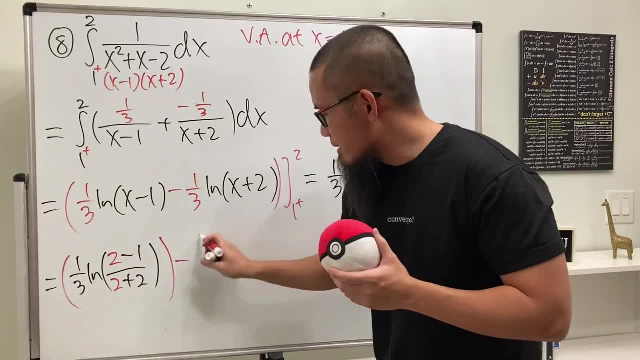 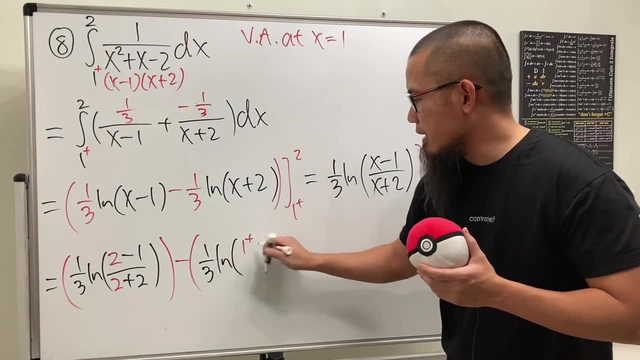 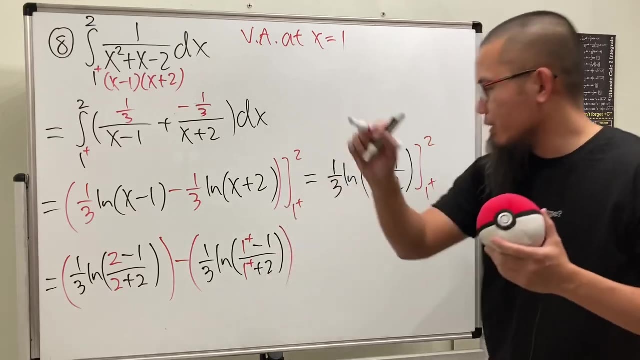 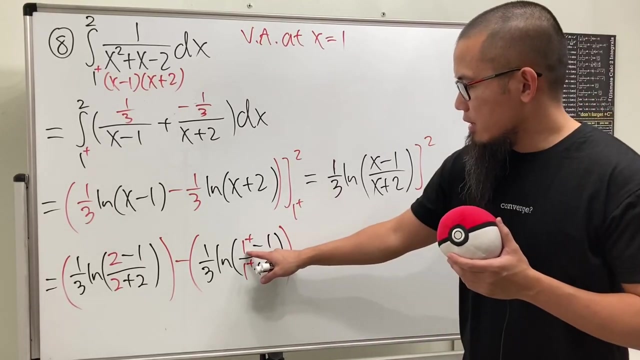 and then minus parentheses. okay, plugging one plus, we get one third ln parentheses. one plus minus one over one. one plus plus two. okay, a lot of work. yeah, i know, but you know what this is finite. let's take a look at what this is. this is zero plus one plus minus one is. 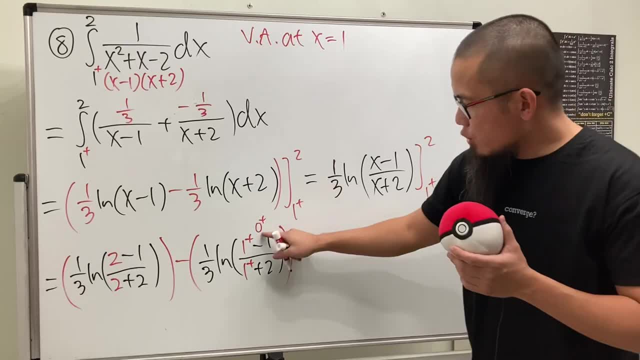 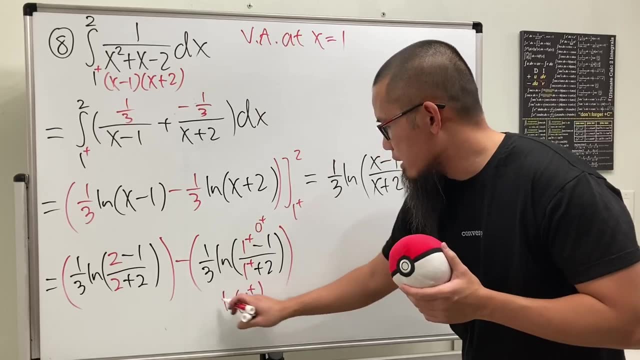 zero plus and again, remember, we're taking a limit. zero plus divided by this is positive, so it's still zero plus. so in fact, here we get ln of zero plus and then we have the one third. but this right here will be the tries got okay and now we got our first number. we do want the second one. so here we are going to get theort from one plus. anyway, we are doing two plus and this is going to get our first zero plus 0 here. so in fact this is going to get our first 1 and third right side, and the third mascara will go into the chicken and make sure That's the sp touching right side, and the second one is going into the fork. there on theأst, put it up: какur 빔CHU. 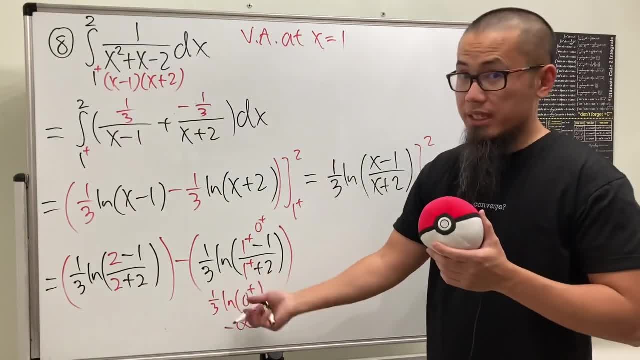 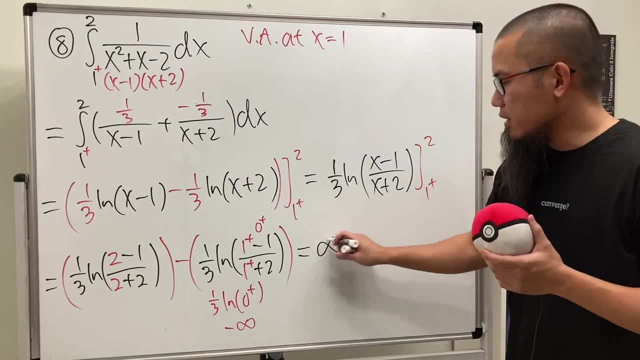 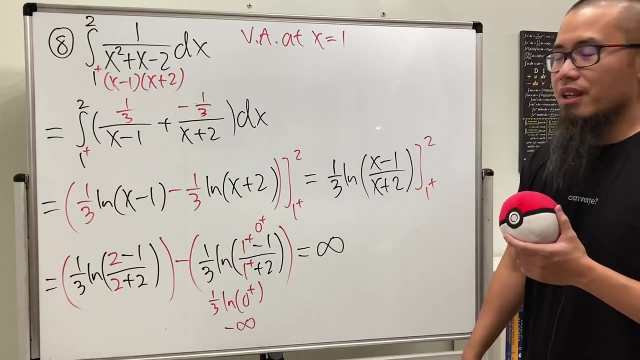 infinity times. one third is still negative infinity, and then negative negative becomes positive infinity. so, in fact, all in all, we get positive infinity. i don't really need to worry about what that is, it's just finite plus infinity. still give us infinity. therefore, you see that that 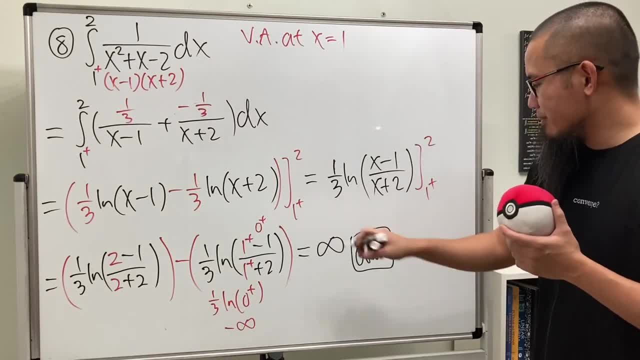 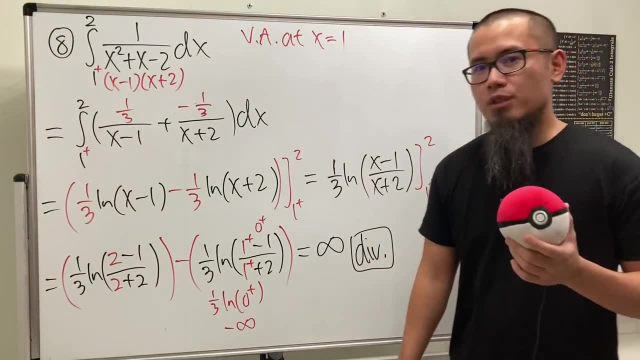 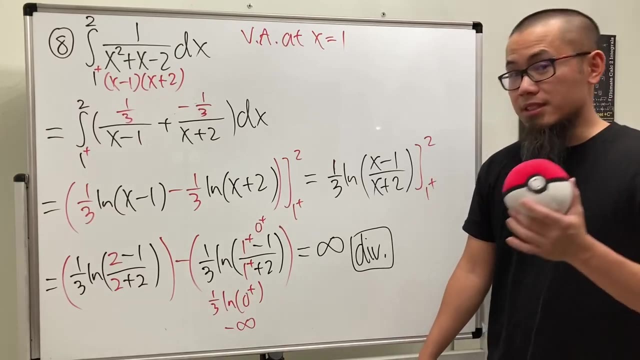 one die purchase and with that we are done. and remember i did a video with the type 1 improper integrals, so if you need to watch that, be sure you click on that video. i'll see you guys there. and if you guys need more help, you guys can subscribe for my channel. you guys can subscribe. 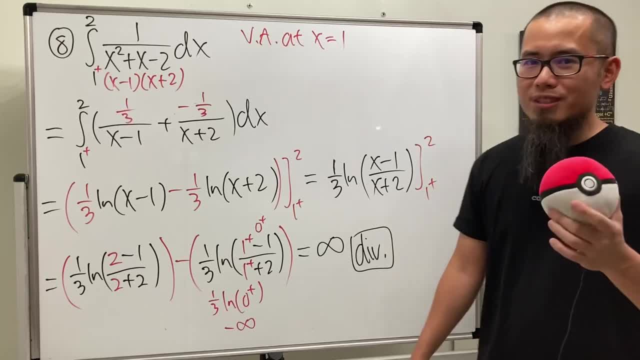 to the channel so that you guys can get the future videos. and, as always, that's it.